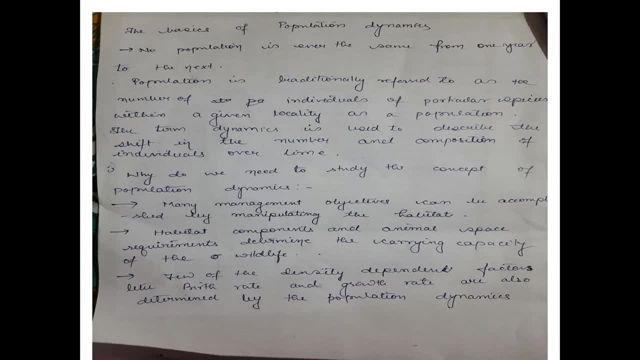 dynamics is necessary to be studied, students, because no population is ever the same from one year to the next. and if we really want to know the status of the population, whether it needs to be conserved, whether it is threatened, we really know to need to know about the population. 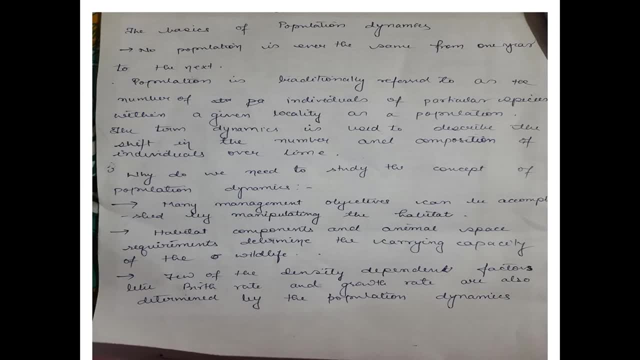 on and home. So study of population dynamics is essential. Population: so let us first know the definition of population. you all have read the different definitions of population right. In statistics it was different. in breeding it was different. now you will say that 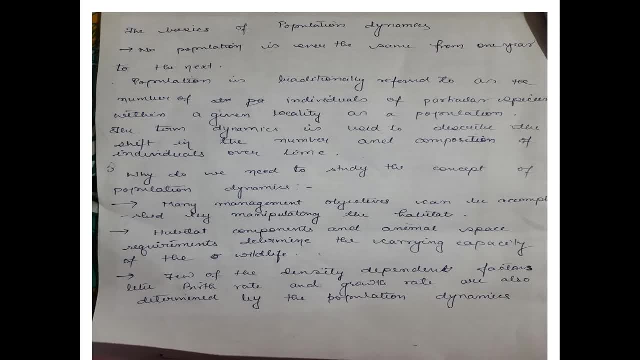 Miami is giving us another definition of population. Well, population is traditionally referred to as a number of individuals of a particular species within a given locality. as a population. The term dynamics, so the together they constitute, population dynamics- Term dynamics- is used to describe the shift in the number and composition of individual over time. and so why do we need to study the 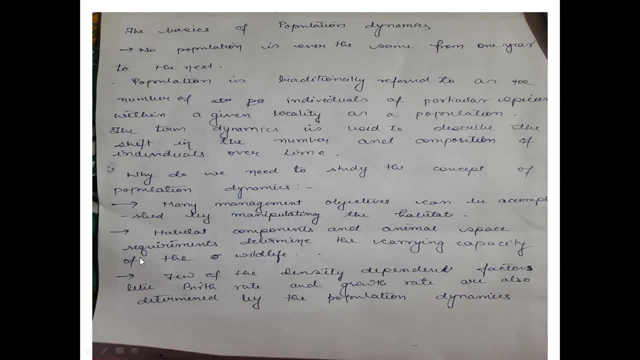 concept of population dynamics. So the concept of population dynamics is used to describe the population dynamics. Many management objectives can be accomplished by manipulating the habitat. So if we want to have many of the managemental works or objectives accomplished, we need to know about the population dynamics. Second, the habitat component and animal space requirement determine. 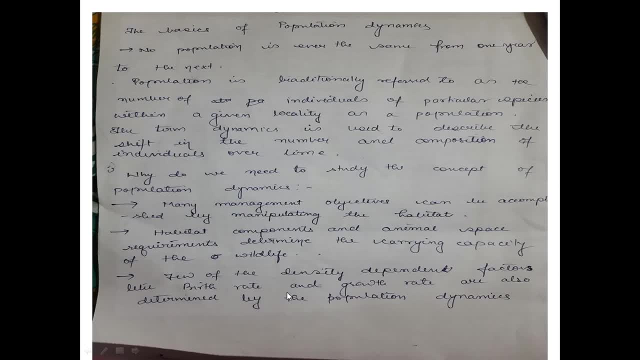 the carrying capacity of the wildlife. and third, few of the density dependent factors like birth rate and growth rate, also determined by the population dynamics. All these terms like density, density dependent, carrying capacity, will be dealt in this lecture, only subsequently. so i would like to explain the concept that. why do we need to study the concept of population dynamics in hindi? 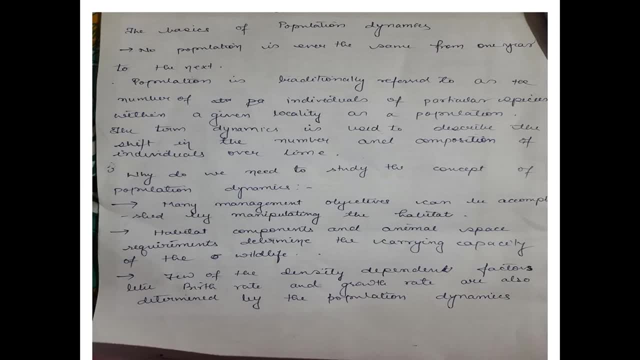 for all of you to understand population dynamics. we need to study population dynamics because dynamics means the different parameters of population taken together: what is the growth rate, birth rate, death rate, what is the density of population emigration, emigration and so on? 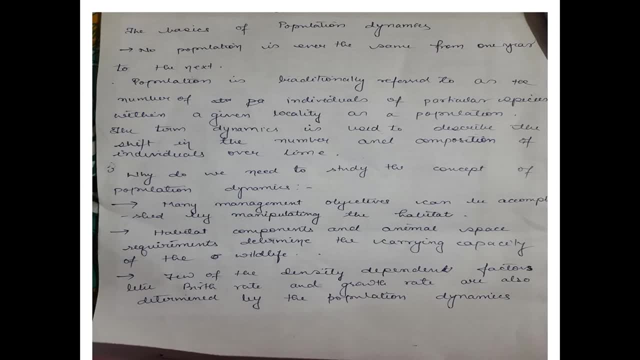 what is the mortality? if we study so many things in whole or part, means we are studying population dynamics. means when we study the dynamics of population, means how much change in population with time or it's number has changed and the composition. when we study this, it justify our knowledge of population dynamics. 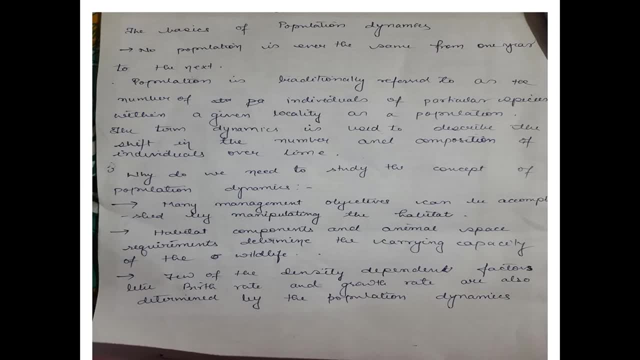 so when we study the change of population with respect to change in its number and composition of individual overtime, we study population dynamics. so when we study the change in population with time, or it's number or position- how much time has taken to change it? So we study it. 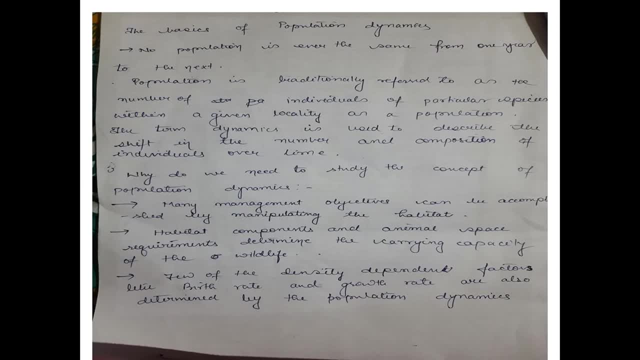 So we study it. So we need to know population dynamics, because if we want to know whether a species needs conservation or not, whether a species is getting extinct or not, then we need to know what is the population dynamics of that species. Second, if we want to know the birth rate or death rate, what will happen next? 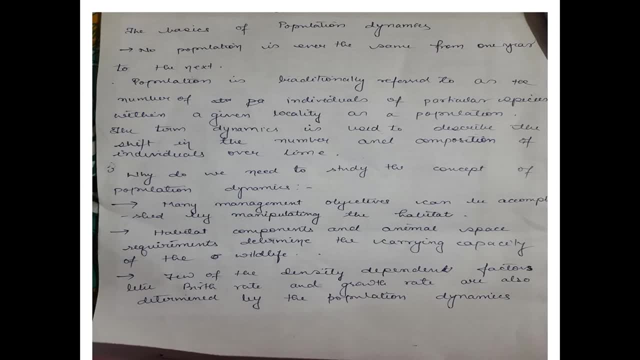 There are many factors, like the birth rate or death rate, of population dynamics that depend on its population, depends on its population density. To predict whether such factors will change over time or not, we need to know population dynamics Overall. the most important point or objective of population dynamics, I feel, is to study. 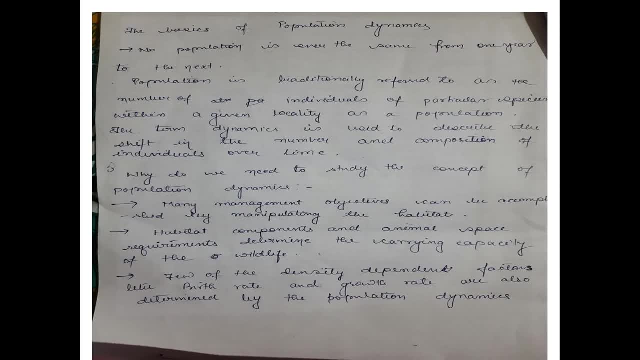 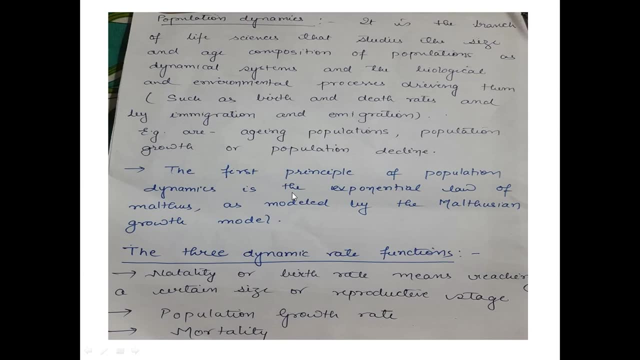 the status of population, whether it is safe or its survivability is safe or not in the due course of time. So we study population dynamics Now. population dynamics over here again. the definition is that it is the branch of life sciences that studies the size and age composition of population as dynamical system. 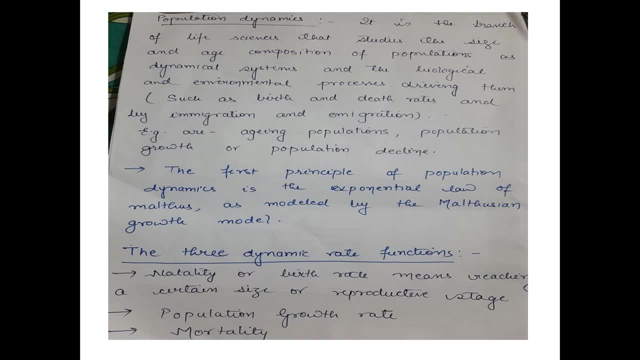 and the biological and environmental processes deriving them, such as birth and death rate, and by emigration and immigration. Well, this definition does look tough. I got it from the literature. It is a concept which has all the meaning. So, explaining it, I would like to say that population dynamics is a branch of life sciences. 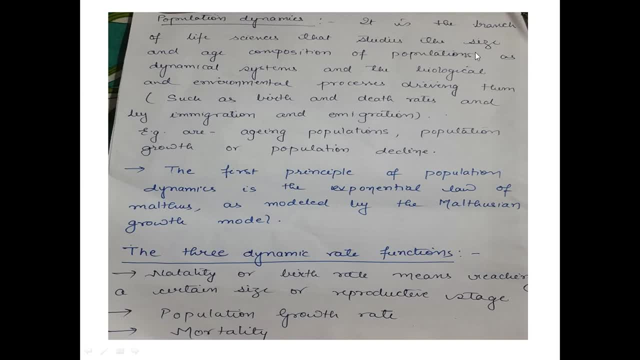 in which we study how much has changed in the size of any population or its age composition, ie how many are of young age and how many are of old age And how many are related to birth rate or death rate or emigration and immigration in. 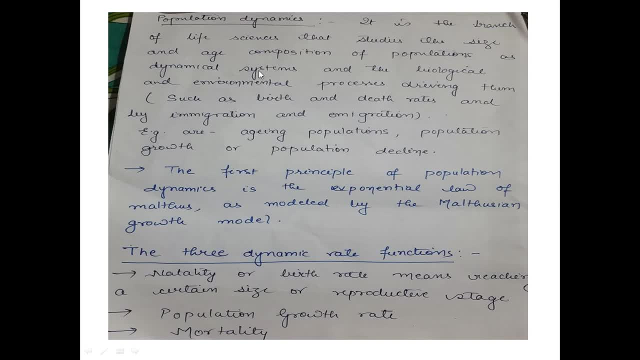 total and how much has changed because of it, its number and composition. So we are studying population dynamics. The first principle of population dynamics to be studied was the exponential law of Malthus, as modeled by the Malthusian growth model. 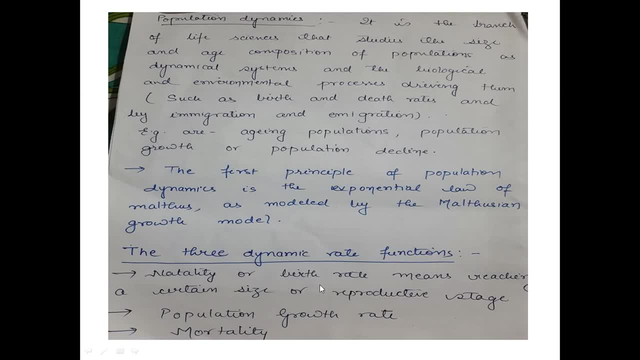 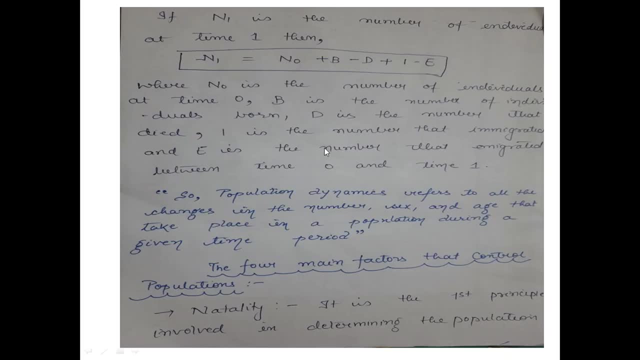 The three dynamic rate functions. natality or the birth rate means reaching a certain size or reproductive stage, population growth rate, mortality. So if n1 is the number of individuals at time 1, ie if we study population dynamics, 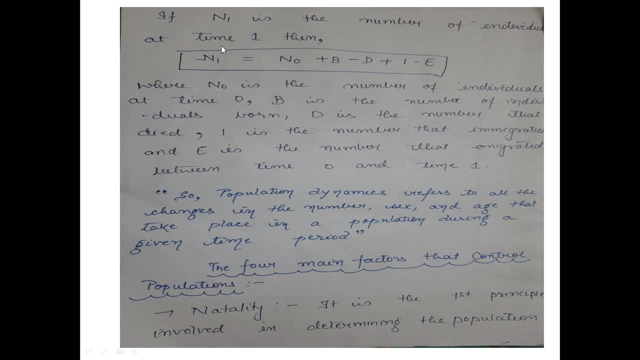 and we want to know the total population. what is its number then? how will we find it? So, at any time, 1,. if n1 is the number of individuals, it will be given at n0.. What was n0 before? 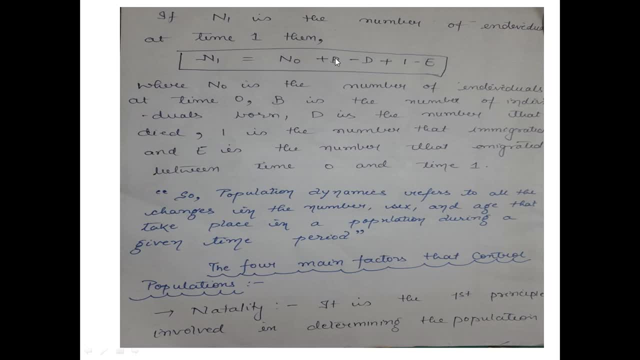 What was its population before Plus b- ie birth, D ie death, I, ie immigration, E, ie emigration, Remember, as immigration is imported from i, ie how many people are there. 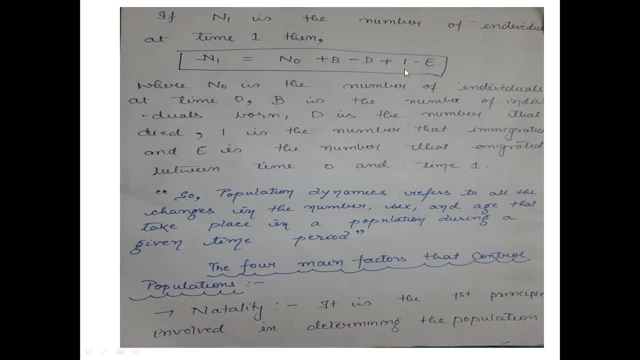 How many animals are there in that population? E means emigration. ie export from. i ie emigration. It means how many animals went out of that population. So what is the number of that population at any time? 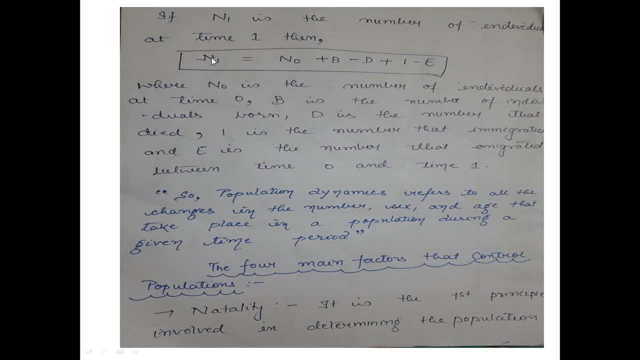 Means. if we want to study the number of resultant number of animals left in a population, we will count it as: how much was it before? N0 plus the new birth taken b minus the death. Obviously it will be minus Plus i, the new entry of animals, minus c the one which who left, the animals who left. 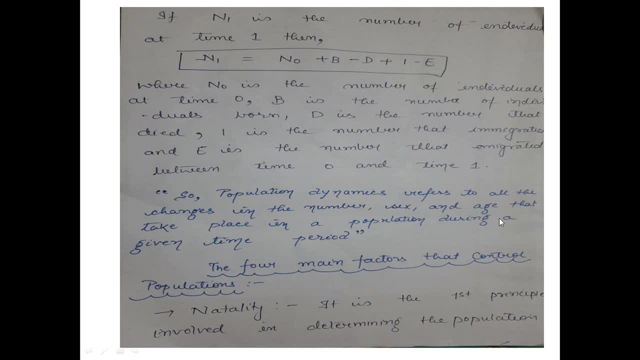 That will give you the resultant animal at any time. So population dynamics refers to all the changes in the number, size, number, sex and age that takes place in a population during given time period. So, student, if I ask you all an objective question in exam, that population dynamics refers to all the changes, or you get this question in competitive examinations. 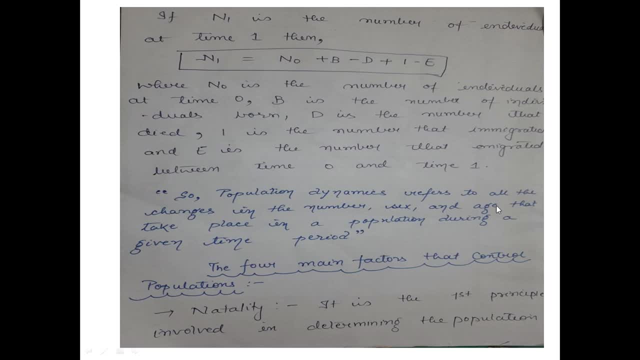 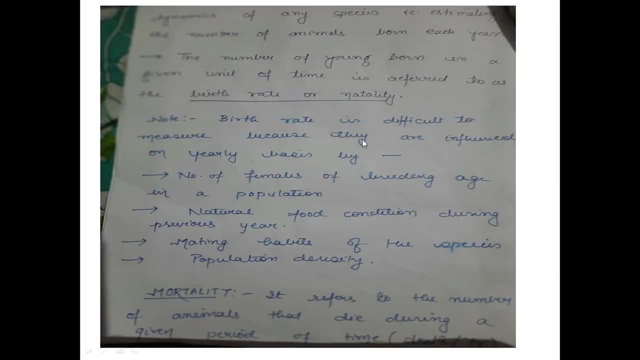 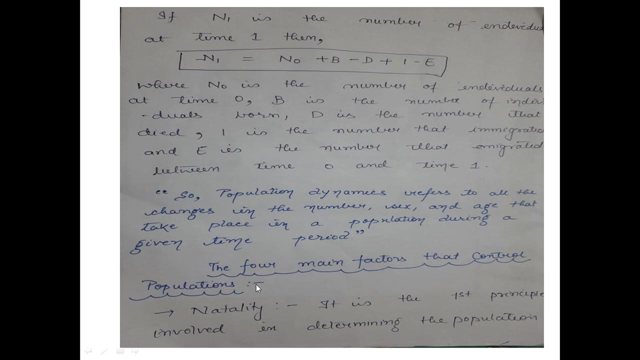 population dynamics refers to all the changes in the dash, dash and dash that take place in population during a given time period. you know what to fill first. Second, if you are asked what will be the formula for N1,, that is, number of individuals at time 1,, then you can say this: 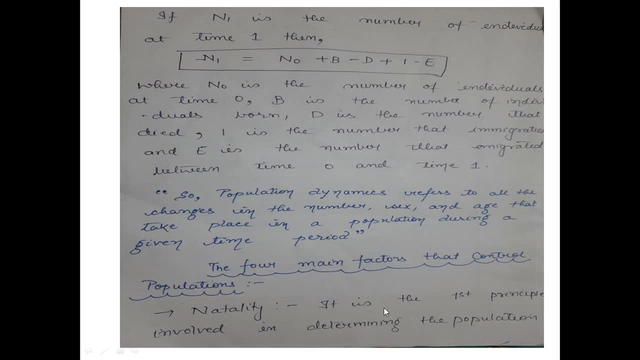 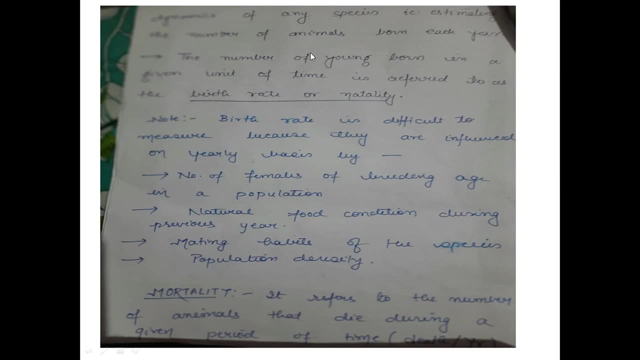 Now the four main factors that control populations is natality. It is the first principle involved in determining population dynamics of any species, that is, estimating the number of animals born each year. The number of young born in a given unit of time is referred to as a birth rate or natality. 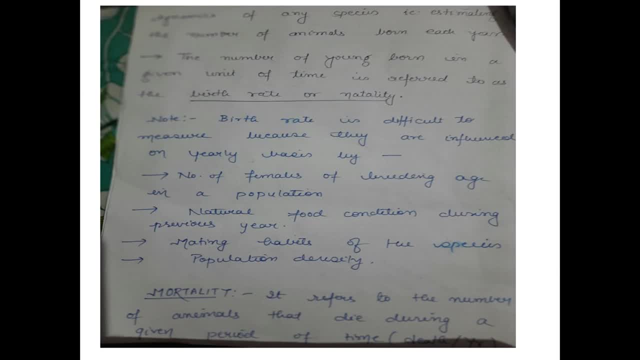 One of the most important and premier and fundamental factors in population dynamics that wevs we study in the parameters in population dynamics is natality. Natality means birth rate. this means how many new animals are born during this time period äch effective as the birth rate or natality. now, birth rate is difficult to measure, although it is the 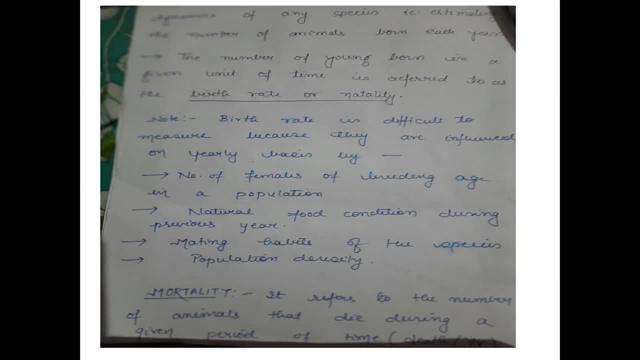 most important factor. it looks easy, but you all can guess why birth rate is rather difficult to be measured in wild animals. in fact, all the population dynamic parameters are rather difficult in wild animals compared to the domestic. or you can understand why birth rate is difficult to measure because they are influenced on yearly basis by number of females of breeding age in 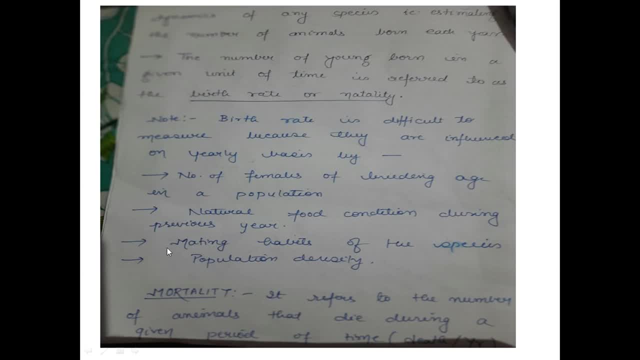 a population. natural food condition during previous year, mating habits of species. population density. First parameter we studied about population dynamics was natality or birth rate. the second parameter, important parameter of population dynamics is mortality and it refers to the number of animals that die during a given period of time. Mortality is of two types. 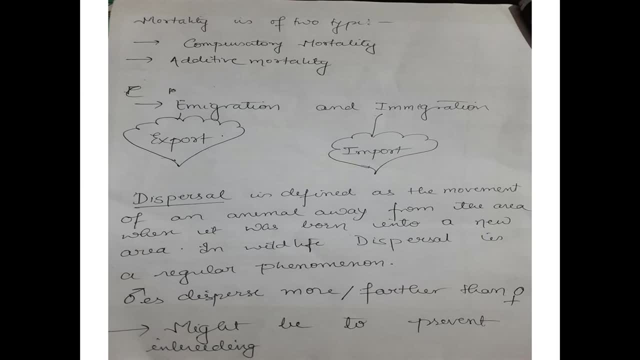 compensatory mortality, additive mortality. how many types of mortality are there? compensatory mortality, additive mortality: what is compensatory and what is additive mortality? before moving on further to the next parameter of population dynamics, which are immigration and immigration, I would like to tell you all that, suppose. suppose in one year death due to disease condition was 25 in a. 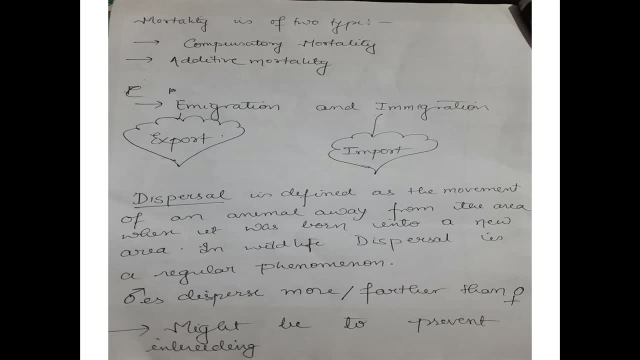 population, 25 percent in a population, while death due, to, say, suppose any natural calamity was fifteen percent in one year, while if suppose second year, in another year the death due to disease condition becomes 35 percent while there is no death due to any natural calamity means overall death will remain constant, 35 percent in both the years. it 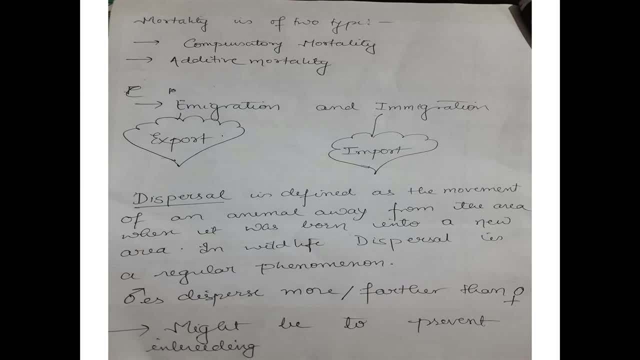 means in this case, mortality due to one cause is compensated by the mortality due to another. this is called as compensatory mortality, whereby the net mortality remains the same. i repeat it once again: if suppose, say, in a year, in an year 2020, in any population, if death due to a disease any 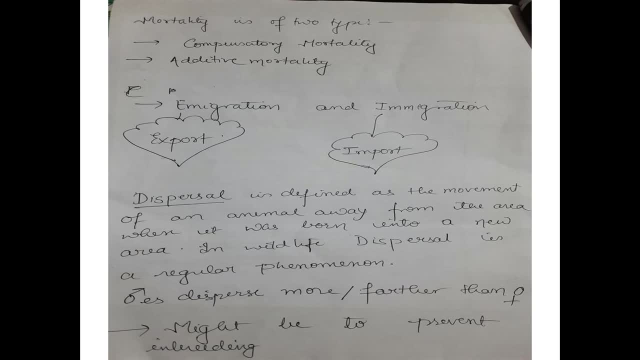 disease condition was 25 percent and death due to any natural calamity was 10 percent and suppose same in same population, the death in next year due to the same two factors, that is, disease condition and natural calamities, are 35 percent and 0 percent respectively. it means 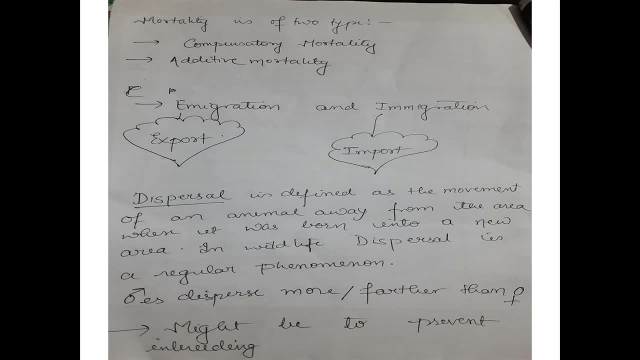 that although overall disease, although overall death percentage, remains the same, it varies for the two factors, but overall remains the same. it means the mortality percentage due to one cause is supplemented by the other or compensated by the other, and this is called as compensatory mortality. but if suppose in another case there is no such compensation, that is, it gets added on. 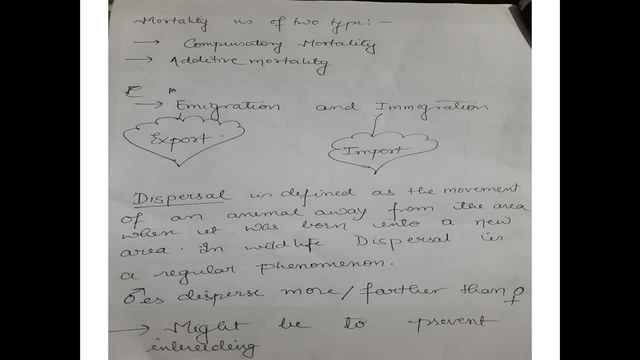 so if suppose in the same popular in a different population in the same year or in different year, death due to disease condition is 25 percent and death due to natural calamity is 10 percent, and in another year death due to disease condition is 35 percent and due to natural calamity is, say, 5, 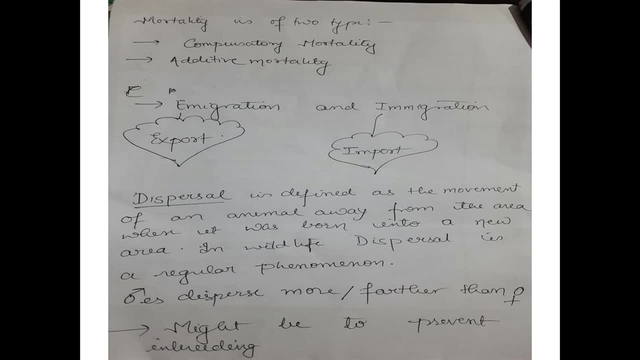 percent, the overall death will increase to 40 percent. so in this condition they are not compensating, but they are adding to the mortality, leading to increased percentage immortality. this is called as additive mortality. let me tell you, in most of the cases, as you can understand the mortality, 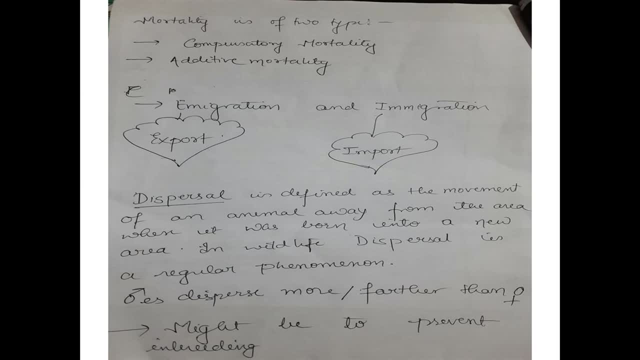 due to the two reasons, are rarely compensated. they are additive in nature. the two another factors, the two last factors, through which four very important parameters for studying the population dynamics are immigration and immigration. so we studied four parameters: first was natality. second was mortality. third, immigration, fourth, immigration. i have already suggested to you all the parameters that we haveo. 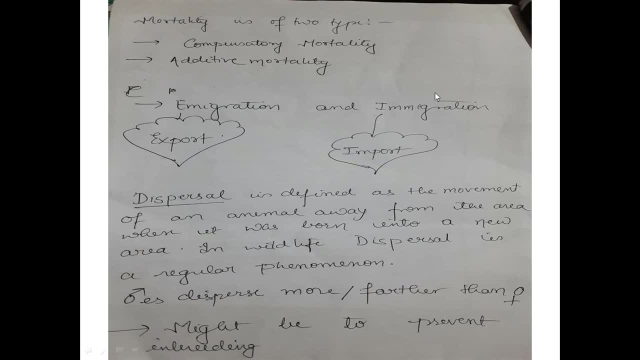 all how to remember it: emigration related to export and immigration related to import. Emigration, similar to export, means export means selling things outside. emigration means when an animal leaves that population and goes somewhere outside. so you can understand that this will make a difference in population dynamics: The age group of animal that has 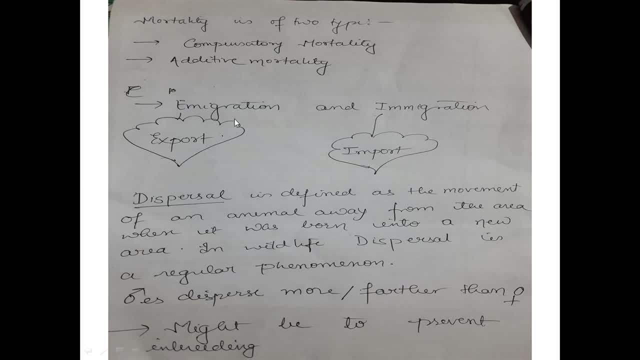 gone from that population. if it is in a low number then it is negligible, but if it has gone in a herd or in a group or in a high number, then population dynamics is bound to be affected. capital N will change capital N1, because if E is more then capital N1 will. 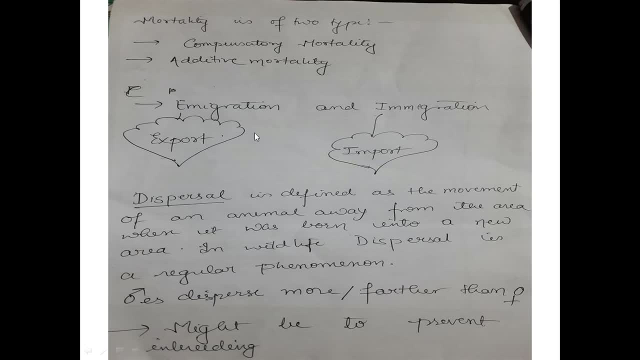 decrease, and especially for that age group who have emigrated more. Similarly, population dynamics will change from immigration. Similarly, immigration is also bound to change the population dynamics depending upon the age or number of animals coming inside the herd. A very important term related to these two last parameters of population dynamics is: 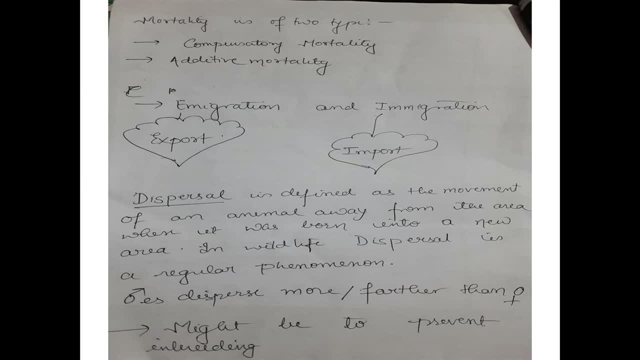 dispersal. Dispersal is defined as the movement of an animal away from the area where it was born into a new area. In wildlife, dispersal is a regular phenomenon. so you might get a question: define dispersal, is it a regular phenomenon In wildlife? yes, it is Increased. 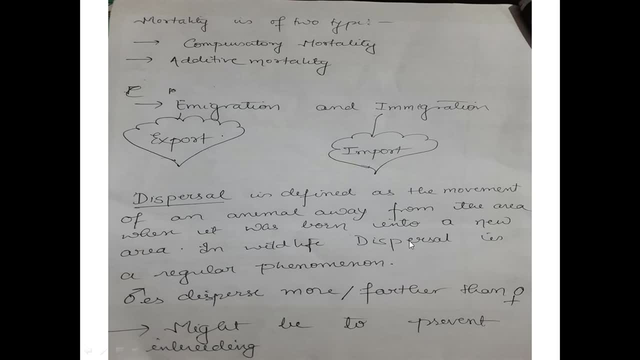 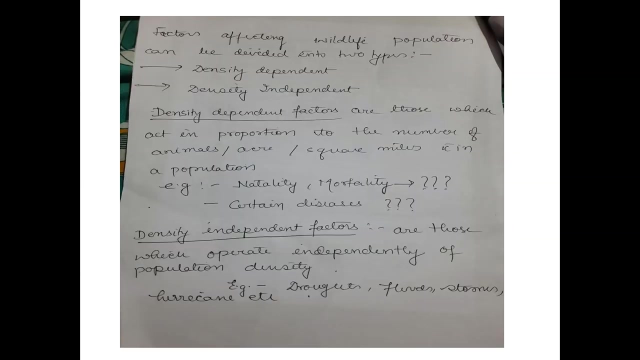 dispersal, so it is also going to change the population dynamics. 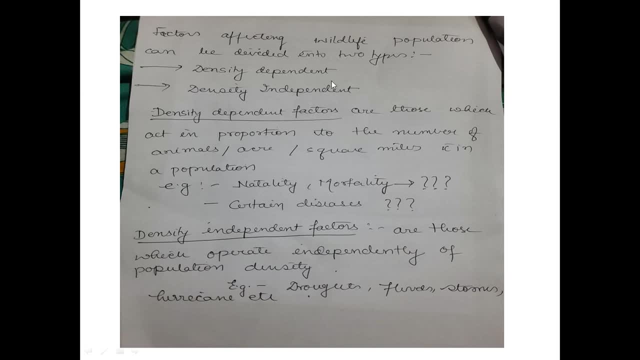 density dependent and density independent. If any of the population parameter depends upon the population density, they are called as density dependent, and if any of the population parameter does not depend on density, it is called as density independent. As you see, density dependent factors are those which act in proportion to the number of animals per acre, per square mile. you know it. 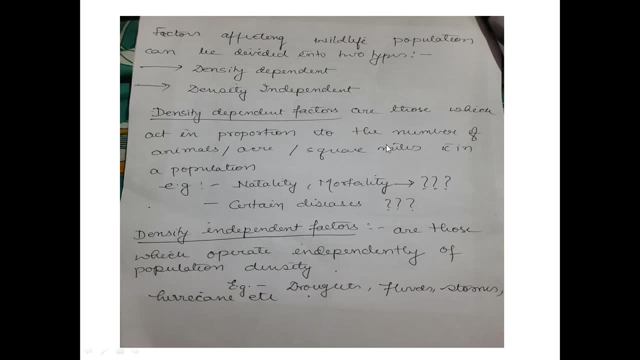 is the population density. ie it means that if there any population dynamics or population parameters which depends upon the density of that population, then we call the density dependent factor. You will know that mortality and natality are density dependent factors. How Certain. 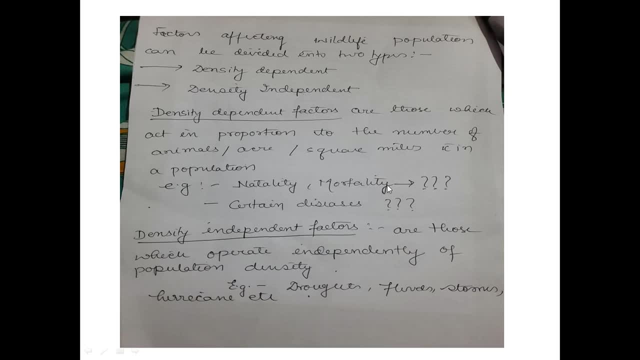 diseases are density dependent factors. How, If the population density in an area is more, If the population density in any ici bhi janvar ki ghanatwa hain, so if the population density in an area is more, they are bound to struggle for food and resources, and so obviously natality will. 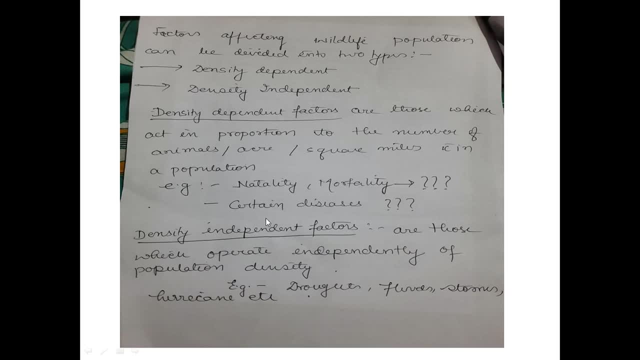 be reduced, mortality will be increased. similarly, certain disease conditions which are contagious or infectious in nature are also dependent upon population density, because they will increase the chances of its spread will increase due to density, population density. so these factors related to population dynamics are actually density dependent factors. opposite to it is density independent. 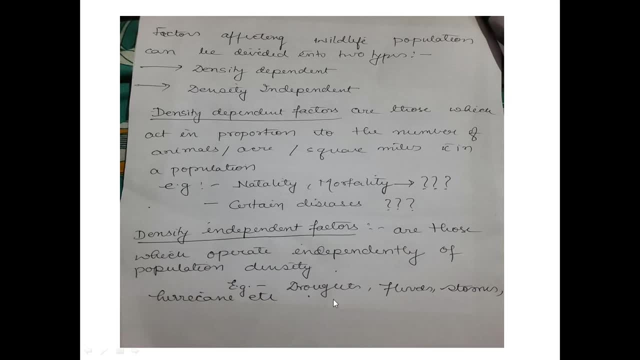 factors which operate independently of population density. example: drought, flood, storm, hurricane. you know they don't ask what is the population density? they are not dependent and this affects the population dynamics. if there is a drought, flood, storm, hurricane, then the number of population is severely affected. 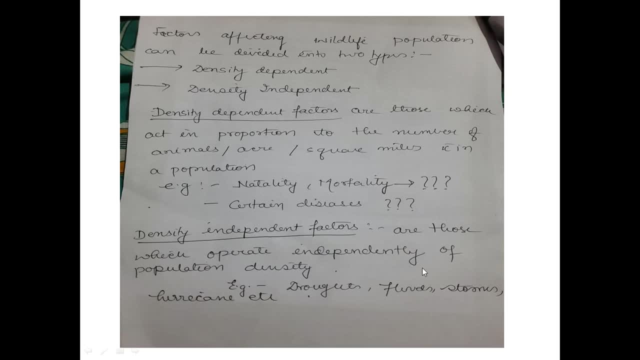 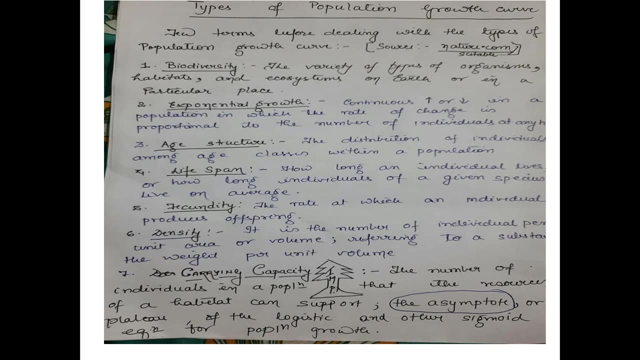 so. so so these factors are density independent factors. now the next topic we will be studying is population growth, types of population growth curves. but before that, few terms which I came across, I took it from naturecom and so I also mentioned the source. so, with due courtesy, so I also would like to describe these terms. what is biodiversity? 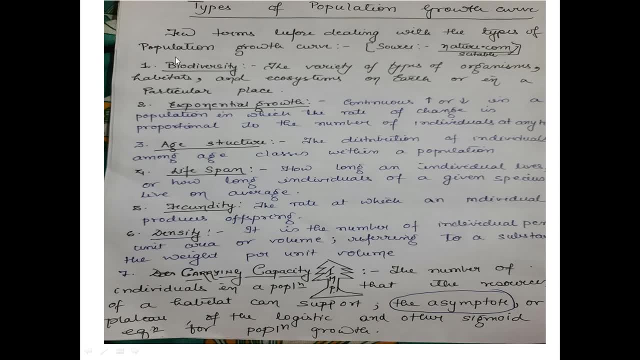 as the name suggests, diversity in the biotic component, that is, the living organisms, is called biodiversity. the variety of type of organisms, habitats and ecosystem on earth or any particular place is called biodiversity. the second term is exponential growth. it is very important. you will come to know that mainly there are two types of growth. 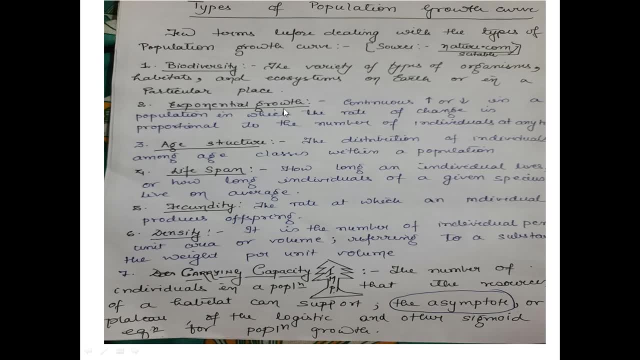 generally, there are two types of growth of the population: exponential growth or logarithmic growth. the first one, as the name suggests, when the continuous increase or decrease in population occurs, in which the change. the first one, as the name suggests, when the continuous increase or decrease in population occurs, in which the change. 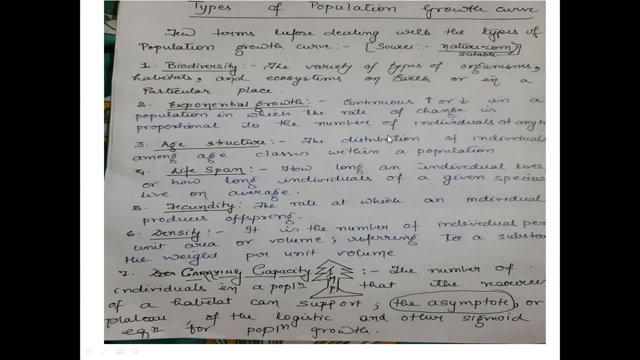 I don't know from where I got it- in which continuous increase or decrease in population is when the rate of change is proportional to the number of individuals at any stage. it is called exponential. the third term is age structure: the distribution of individuals among the age classes within a population. 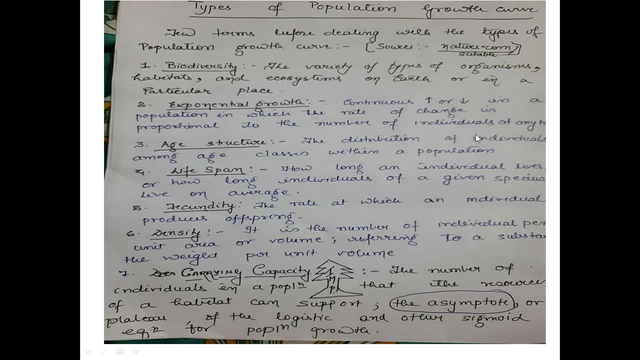 when we divide a population by its age, based on age, we call it as age structure. when we divide the population into different ages, the lifespan- how long an individual lives. the lifespan, how long an individual lives, you know, it is but a very common term. Fecundity: the rate at which an individual produces offspring. 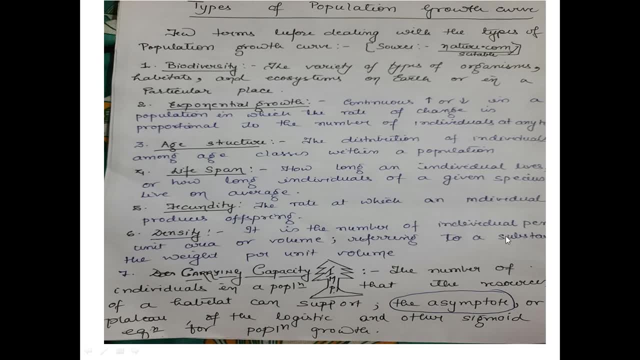 related to fertility, prolificacy. Density: it is the number of individual per unit area or volume referring to a substance. the weight per unit volume. Carrying capacity is an important term. I have written IMP for important, So do remember it. You might get a definition. what is the carrying? 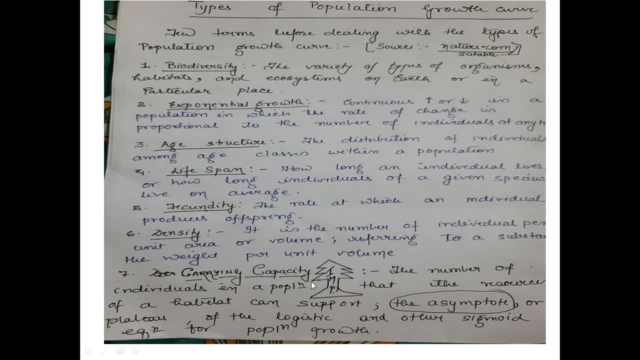 capacity Carrying capacity. friends, when you go for any webinar meeting, in few of the Zoom they say hundred, hundred limit has been reached. So sorry, we cannot give you entry. The host does not give you entry and you are not able to attend the webinar. So the carrying capacity of that? 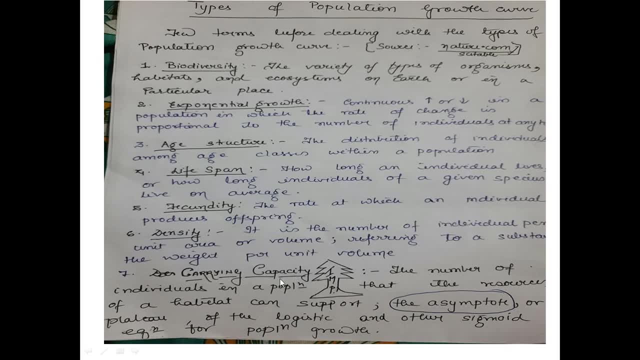 webinar is hundred. Similarly, the nature also has its carrying capacity: for the animals, for the human, for its inhabitants. It is the maximum limit to which it can let the human or animal sustain. So the number of individuals in a population that the resource of a habitat can support. 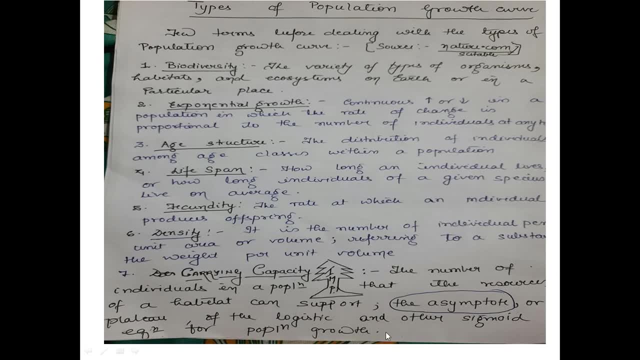 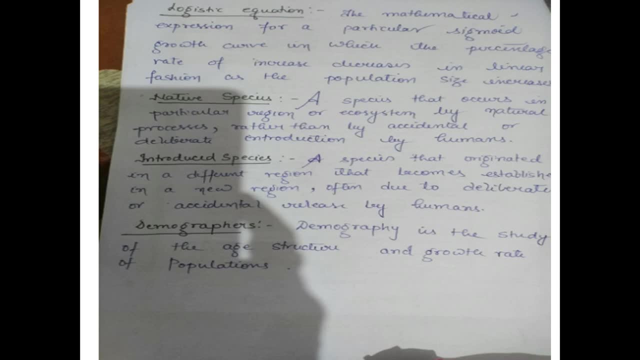 the asymptote or the plateau of the logistic and other sigmoid equation for population growth. Not making it rather difficult, I would like to say the carrying capacity is the maximum limit. A maximum limit a particular place or the natural resources of a place sustains. 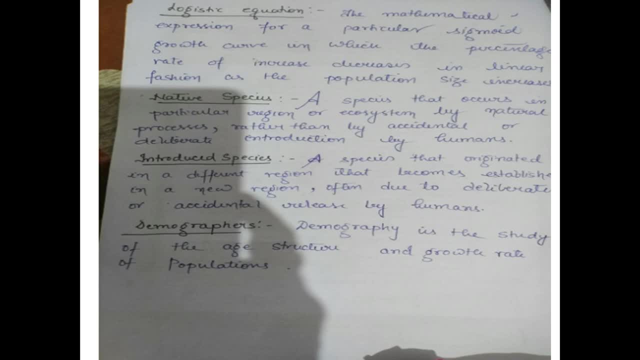 with respect to the number of animals, or human, is called the carrying capacity. Logistic equation is the second type. One was exponential. another is a logistic equation, Mathematical expression for a particular sigmoid growth curve in which the percentage rate of increase decreases in linear fashion as the population size increases. We will be studying. 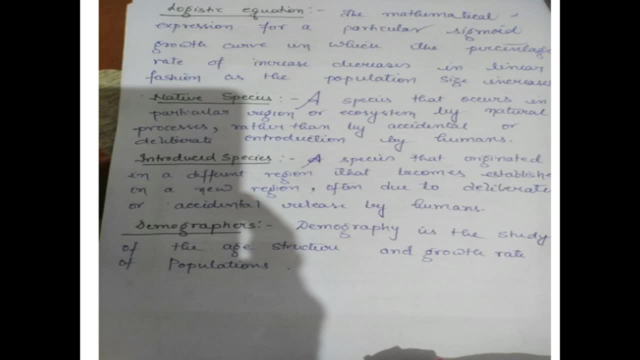 it right now: Native species, a species that occurs in particular region or ecosystem by natural process, rather than by accidental or deliberate introduction by human. So if suppose an animal or a particular species that occurs in a particular region or ecosystem by natural process, one is the native species In a particular area and in a particular place. you find Ohi. 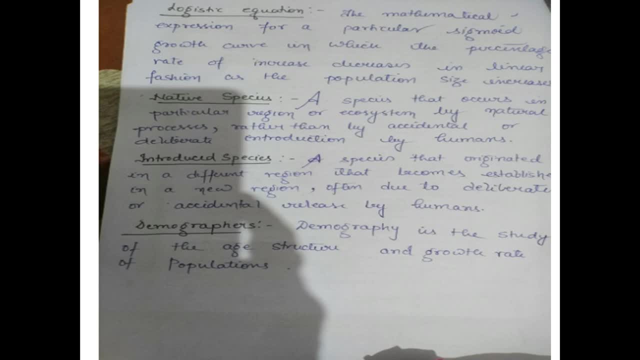 it is the native species, the in the natural inhabitants of that place. this place we call it as native species. In few of the fields you find the weeds like manure, growing by itself without any seeds or anything. So you say that it is the native. 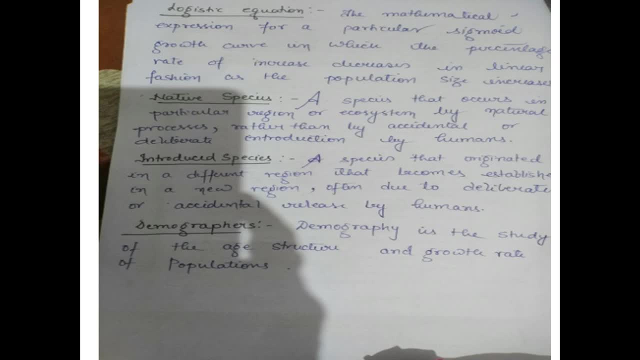 species of that place, In a pond or particular area, particular, you will have particular animals always there without any of the human intervention, in that they are natural species. So someone gathered At the meeting task of aité. It's my position to know that the dzikora is bitte, You must know this. Just type in long PHEW participates. I don't know that I have to take a few seconds to process that. tomato Inbuild is Parlament locally and in La Ruta. 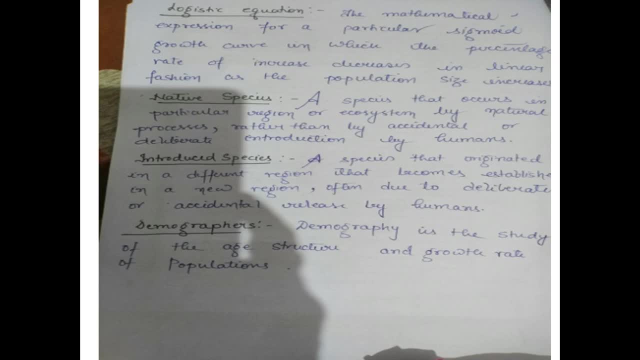 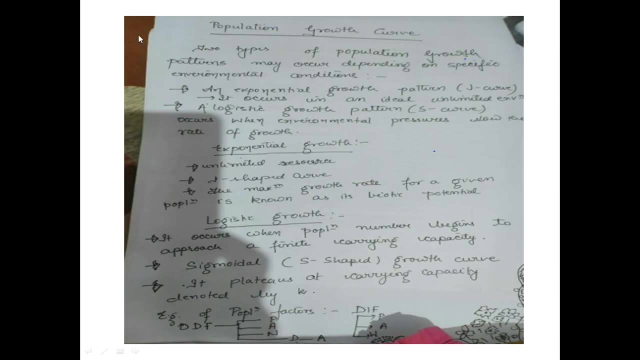 Does it世界 a traditional plant species or in the neighborhood N Same w that you decide that we are interested? Contrast to it are those species which are actually introduced or deliberately into that regions. and demography is the study of age structure and growth rate of a population. Now coming to the main. 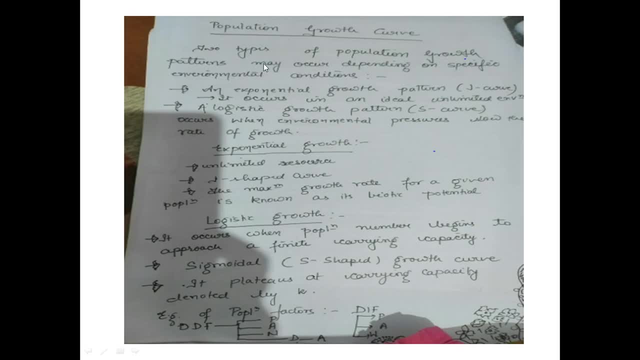 heading, that is, population growth curve. It is very, very important. two types of population growth patterns occur, depending upon specific environmental condition. I would like to add to it ki environmental condition ke saath saath type of population pe bhi depend. karta hua do tarah ke. 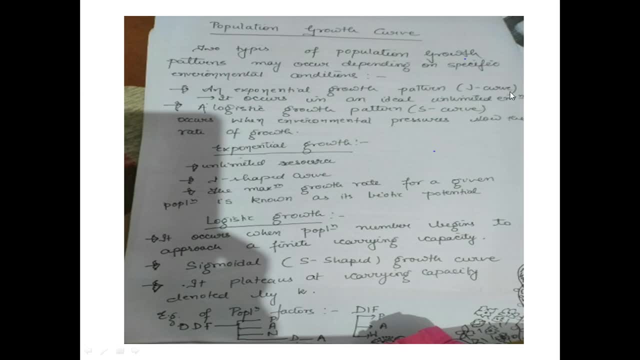 growth curve pae jaate hain. ek exponential growth curve pae jaata hai, jisko hum log j curve bhi bolte hain. ye ek ideal unlimited environment me hota hai, jisme ki unlimited grow karta hai. population, jisko ki hum log exponential growth curve bolte hain. Wahi dosra tarah ka hota hai logistic. 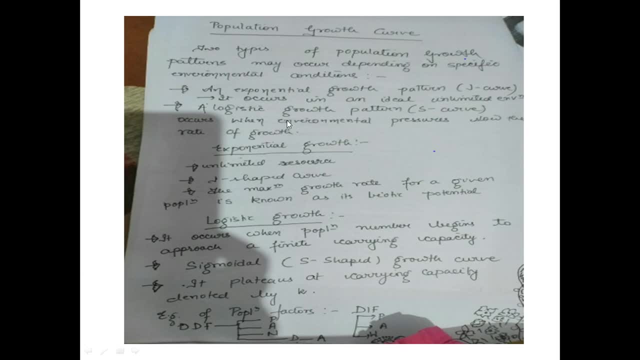 growth curve. jisko S curve bolte hain, ya sigmoid curve bolte hain. it occurs when environmental pressure slow the rate of growth. Agar hum log human ki baat kare to they j or the mammal, they show S curve. or any other curve they show S curve. So it occurs when the growth curve is. 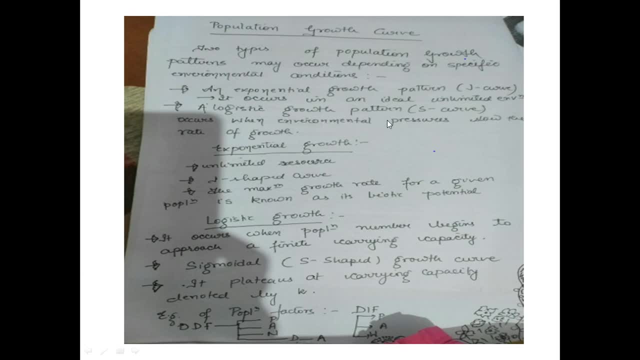 very, very high and the animals generally show S curve whereby it increases to a limit and then starts decreasing as soon as the carrying capacity is reached. Matlab ek limit ke baat. the growth rate is reduced, stopped. it is called as a logistic growth curve, Now exponential growth curve. 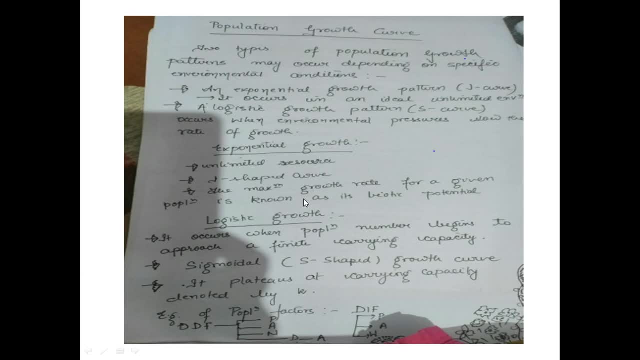 few features: unlimited j, so j shaped curve. maximum growth rate for a given population is known at now an important term. the maximum growth rate for a given population is known as its biotic potential. So if you are asked, what is the biotic potential any population's? 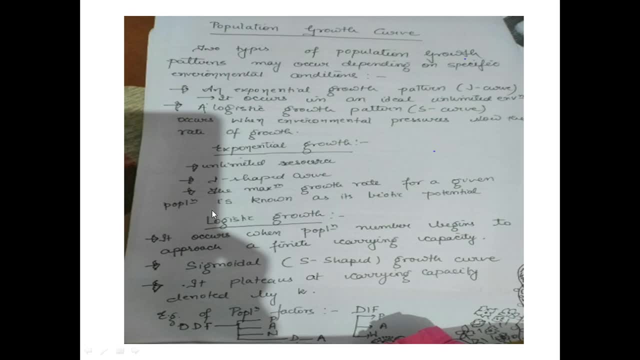 maximum growth rate is its biotic potential. Now the second type of curve is logistic growth curve. It occurs when the population number begins to approach a finite carrying capacity. It does not have infinite growth, unlike exponential. As I said, after carrying capacity it starts to decrease. or it will be reduced or it will be constant- Sigmoid. 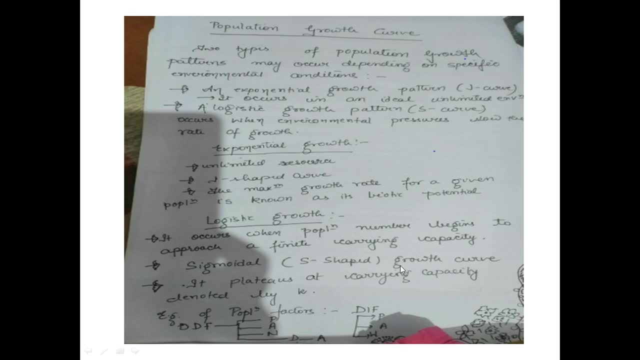 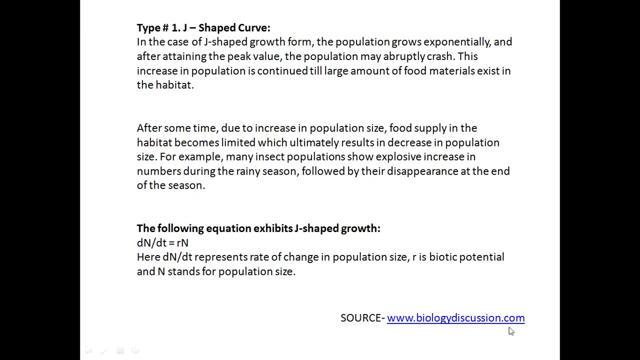 growth curve. its plateau at carrying capacity is denoted by K, First one. now, in detail, the same thing. the source: wwwbiologidiscussioncom, with courtesy: Type 1 is J-shaped curve. In this case of J-shaped form, the population grows exponentially and after attaining the 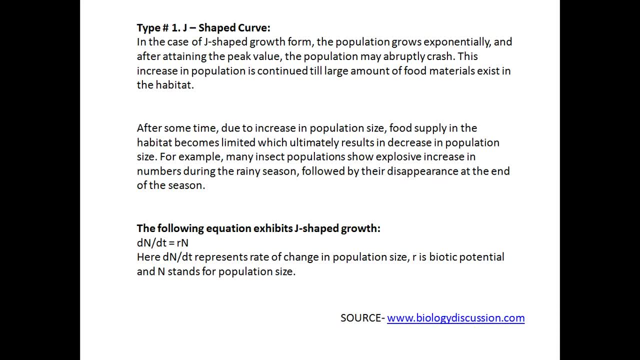 peak value, the population may abruptly crash. This increase in population is continued till large amount of food material exist in the habitat. So in case of J-shaped curve, for exponential curve it is rather unlimited, but it might happen at a particular point. 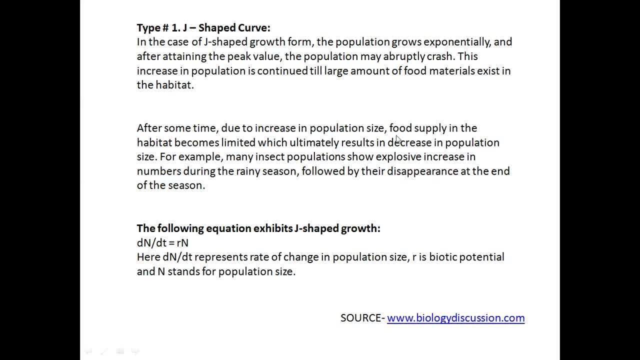 it suddenly stops the growth or it crashes After. sometimes, due to increase in population size, the food habitat becomes limited, which ultimately results in decreased population size. It is mainly observed in many insect population, which shows explosive increase in number during the rainy season, followed by their disappearance at the end of the season. So here you get the example of exponential or the exponential growth curve. So you get the example of exponential or the exponential growth curve. So here you get the example of exponential or the exponential growth curve. So you get the example of exponential or the 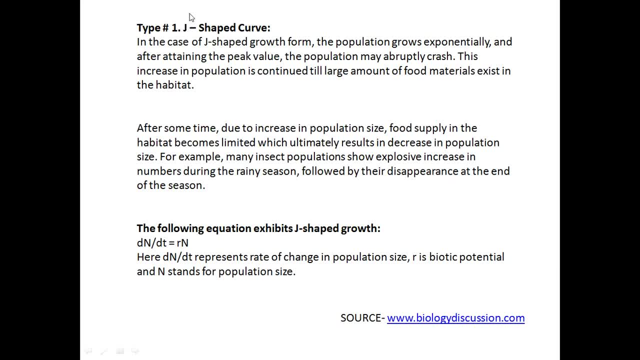 J-shaped curve. As you can see, J-shaped curve- the first type of curve is called J-shaped curve, which is generally called as an exponential curve, which generally has unlimited growth. It may crash after a certain point of time, but after increasing it never has a decrease. 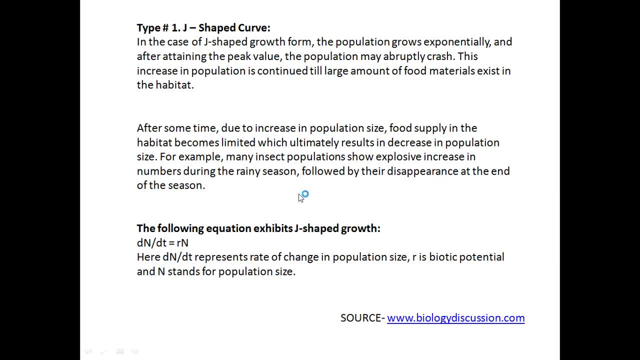 as in sigmoid, and it can be observed as in small insects and very small animals. The equation of this J-shaped curve is: DN upon DT is equal to Rn. That is the rate of growth rate of differential. this is the differentiation: dn upon dt is equal to rn. So rate of increase. 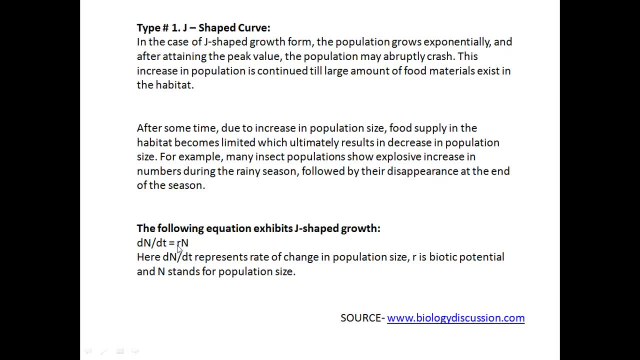 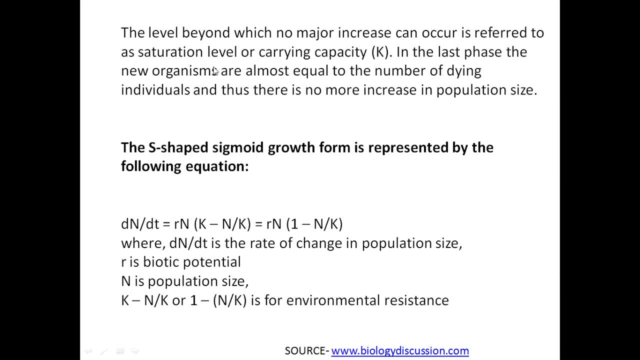 of population is rather dependent upon r, the biotic potential, and n, the population size. Now the level beyond which no major increase occurs is referred to as saturation level or carrying capacity, which I have already said. In the last phase, new organisms are. 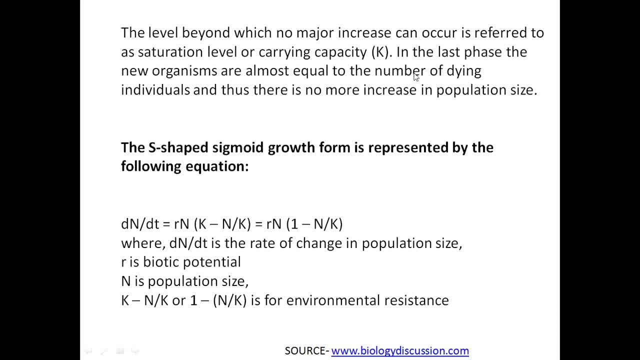 almost equal to the number of dying individual, and thus there is no more increase in population size. The second type of growth curve is S-shaped sigmoid growth form, which is represented by following equation: dn upon dt is equal to rn into k minus n upon k, which is equal. 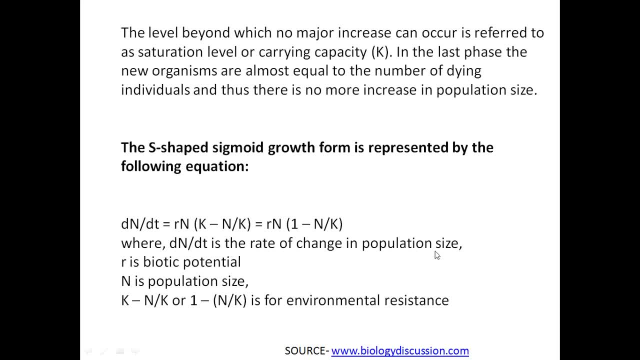 to rn into 1 minus n upon k, where dn upon dt is the rate of change in population size, r is the biotic potential, n is the population size, k minus n upon k, or 1 minus n upon k is for environmental resistance When a few organisms are introduced into an area, the 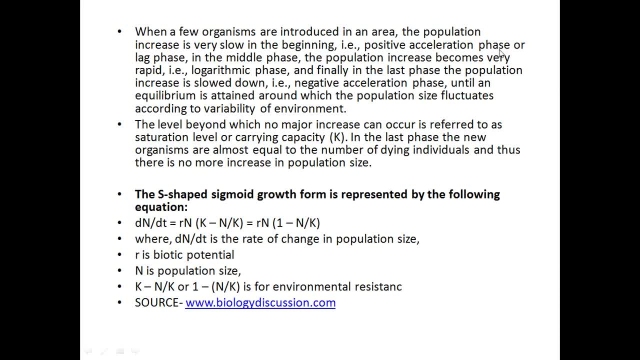 population increases. This is very slow in the beginning. That is positive acceleration phase. These are the phases of sigmoid curve. Just now we will be explaining it, first of all through a theory and then by graph. In exponential growth curve there is no such phase. It increases continuously. 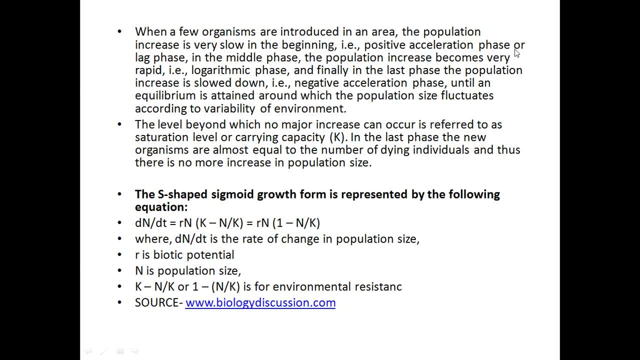 But in sigmoid curve or S-shaped curve. first we get to see positive acceleration phase or lag phase, when growth is a little slow. In the middle phase population increase becomes very rapid. We call it logarithmic phase. And finally, in the last phase, population increase is. 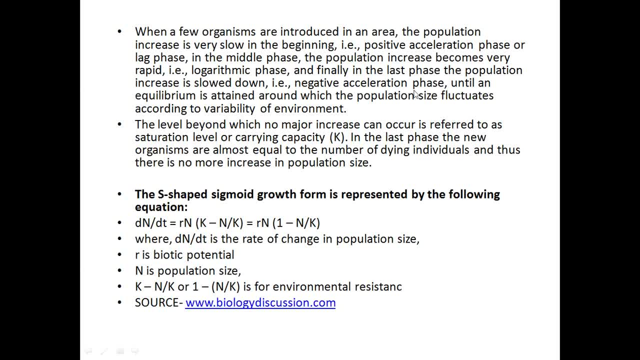 slowed down- We call it negative acceleration phase- And it goes on until an equilibrium is attained around which the population size fluctuates according to variability of the environment. The level beyond which no major increase can occur is referred to as saturation level, or carrying capacity. In the last phase, new organisms are almost equal to the number of. 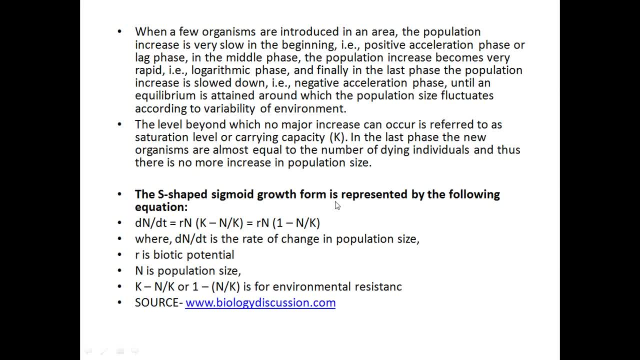 dying organisms. Thus, there is no more increase in the population size. The S-shaped sigmoid growth form is represented by the following equation: This is the equation for S-shaped sigmoid growth curve. As you can see, in this case the growth rate is dependent upon the carrying capacity. K. 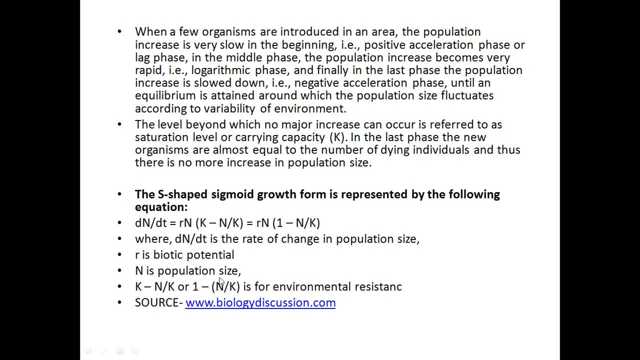 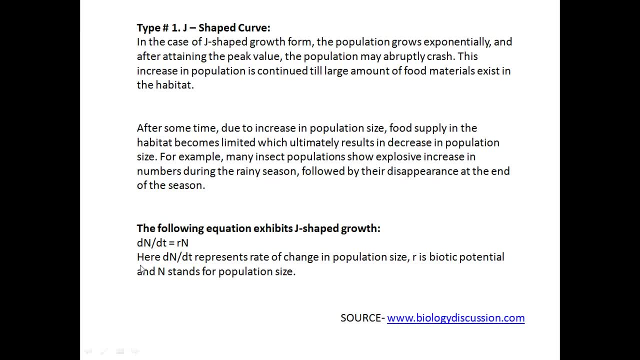 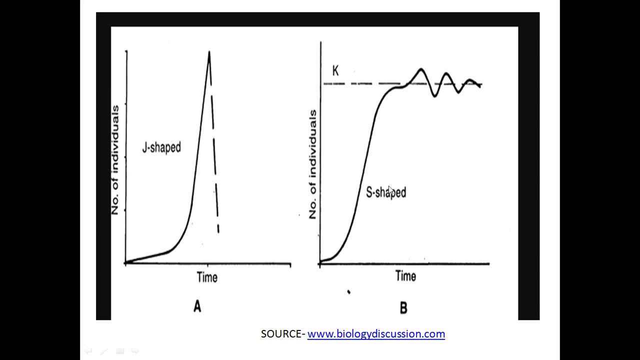 the biotic potential, R and N, the population size. But in this case it is in case of the sigmoid growth J-shaped curve- it is dependent only upon the carrying capacity. So these are the two curves. As you can see, this is the J-shaped curve. So, if you are, 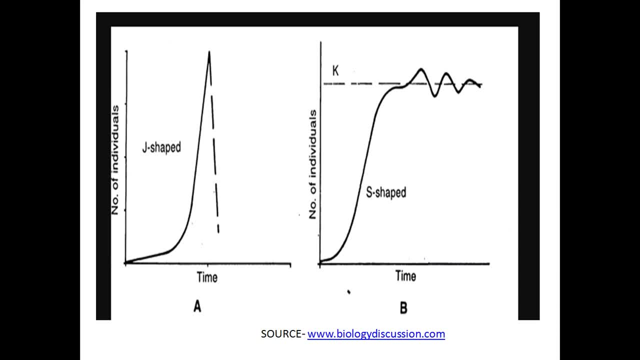 asked what are the different types of population growth, you can say they are basically of two types: J-shaped or exponential, S-shaped or sigmoid. So if you are asked what is the basic difference, you say that in case of J-shaped curve or exponential growth, it increases. 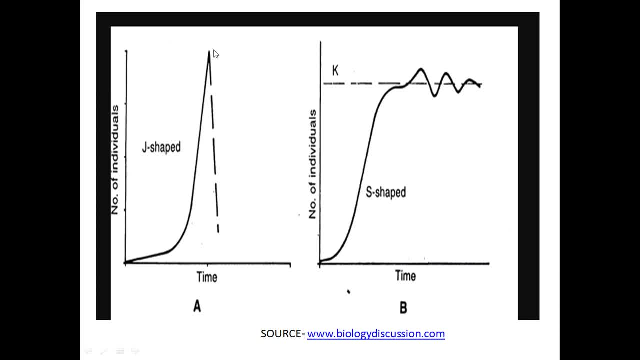 infinitely, after which it might crash. But up till that there is no log phase or lag. There is no lag phase or deceleration phase. It increases infinitely. While in case of S-shaped curve, you have a lag phase where the growth is slow, You have a log phase where 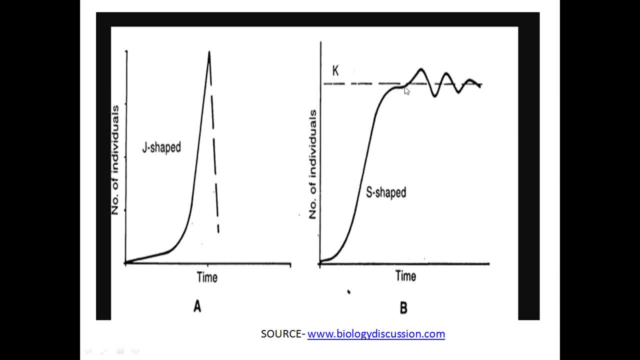 the growth is very fast, and then you have a negative acceleration phase whereby it almost becomes constant, and then it increases or decreases at the equilibrium, depending upon the carrying capacity. K: This J-shaped curve is not dependent upon the carrying capacity. as it increases, It increases infinitely. Let me tell you: when practically most of the population show 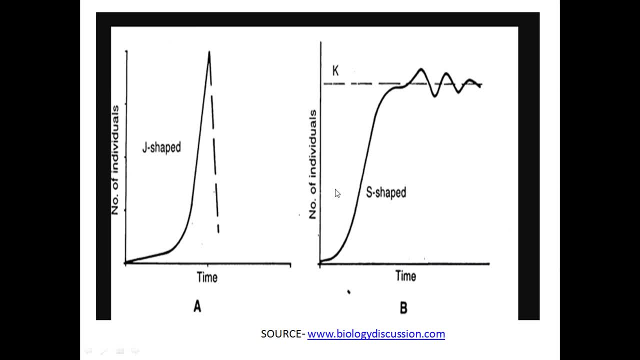 this curve, that is, S-shaped curve, because after a limit, definitely the carrying capacity of the resource of the nature will be reached, There will be a shortage of food supply and then there cannot be an increase beyond that, While this J-shaped curve is noticed in case of insects. so there was an example of this. 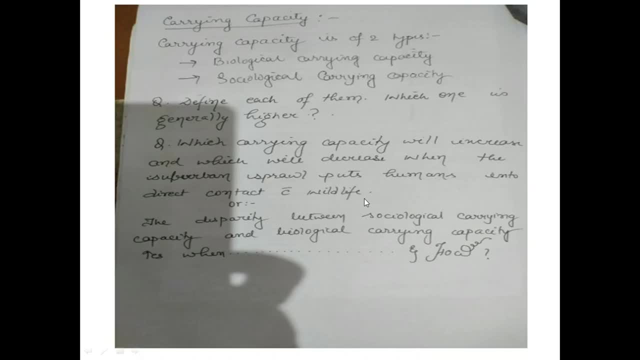 and this. These are the meist common MOVs and we have found that in such a world, indeed, we have also found that in the world, there is a WOVs, as we discussed it Now, carrying capacity. This term is encountered at many places, so let us see. 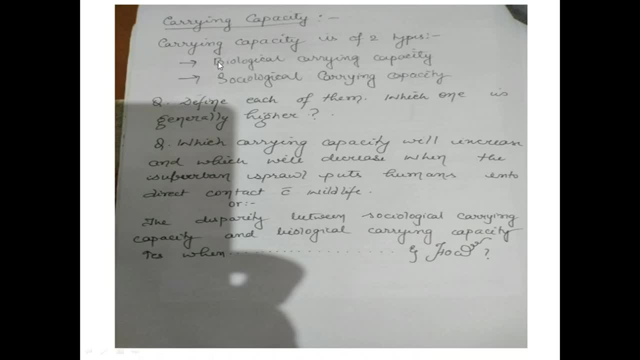 Let me tell you all this: biological carrying capacity is the carrying capacity of the nature or the natural resources, and sociological carrying capacity is the carrying capacity with respect to human Means. how much can we tolerate the animals and biological animals are vulnerable and we can't tolerate them. 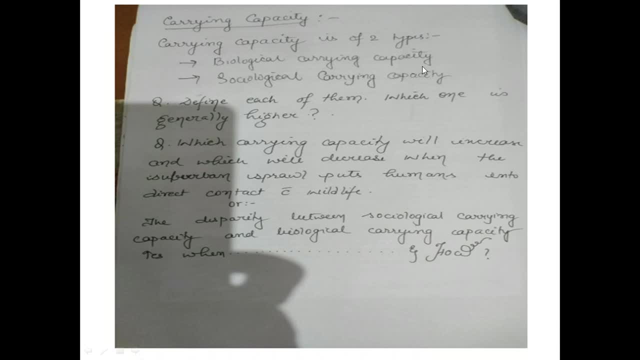 So the very basic question that we have to answer is whether or not the biological animals are Biological. carrying capacity is: how much can the nature tolerate? So these two are very, very important. Now, if you are asked, define each of them. which one is generally higher? you know, define. if you compare both of them- biological carrying capacity and sociological carrying capacity- generally, biological carrying capacity is higher than the sociological carrying capacity. It means the limit of maximum animals nature can tolerate or sustain is called biological carrying capacity, and the maximum number of animals we can sustain or tolerate we human. 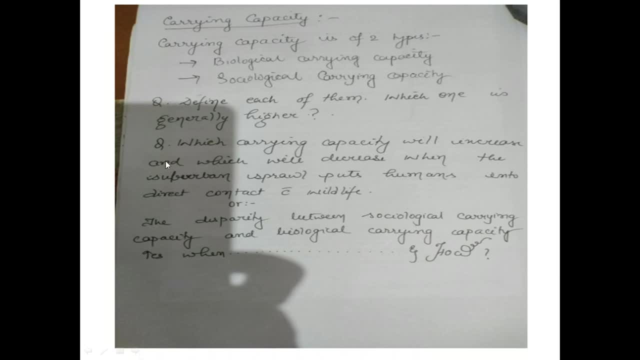 are called sociological carrying capacity. Which carrying capacity will increase and which will decrease when the suburban sprawl puts human into direct contact with wildlife, Say, suppose we- this is witnessed most of the times when, we suppose, invade the habitat of wildlife Due to increasing population density, we are definitely having human intervention and human 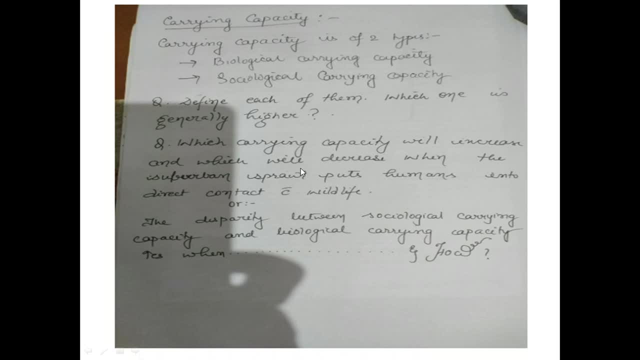 population settled almost everywhere. So when it starts at say, suppose at a place which was earlier inhabited by wildlife, you know, although the biological carrying capacity will increase, the sociological carrying capacity will decrease. Why biological carrying capacity will increase. 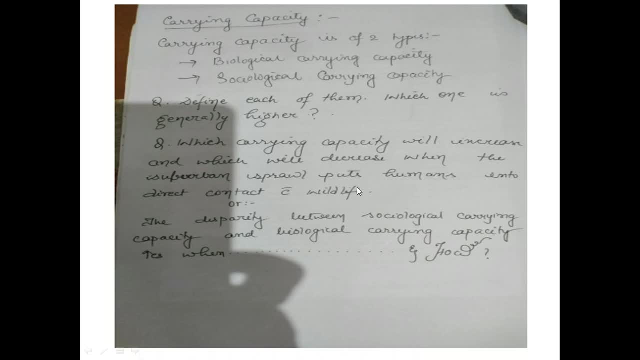 Because the wild animals in the vicinity of human will be supported by the natural food as well as the food, waste And all from the human. But then, because the human has now settled to the nearby, it will try to reduce the habitat of the wildlife and so sociological carrying capacity will decrease. 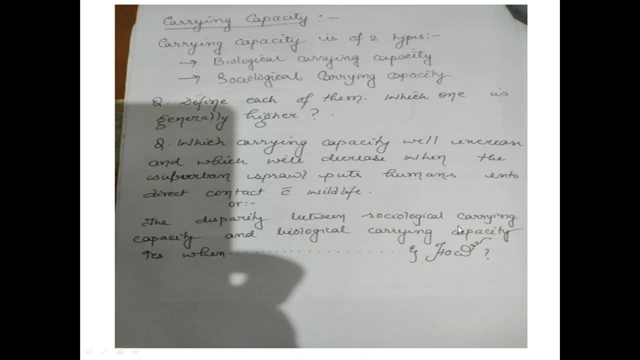 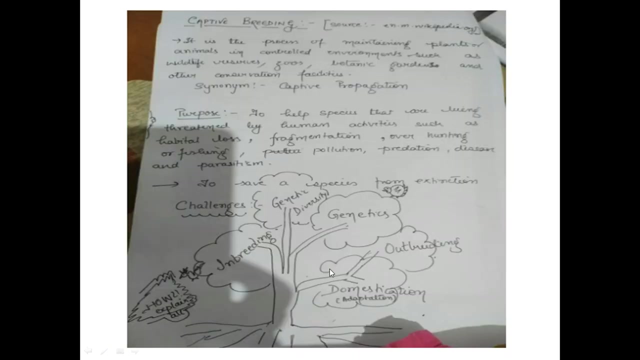 The disparity between it is a very important question. the disparity between sociological carrying capacity and biological carrying capacity increases when you get the answer here. increases when the suburban sprawl puts human into direct contact with wildlife, and how I have just now explained. 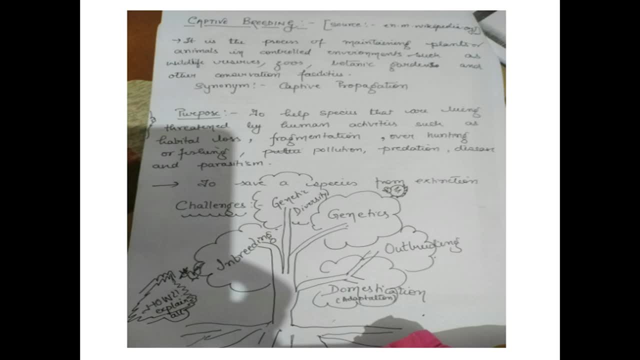 Now, coming to the term captive breeding. it is very, very, very important. This captive breeding, as the name suggests, is breeding in captivity. It means if we get it captive in a zoo, or if we get it captive in a prison. we call it. 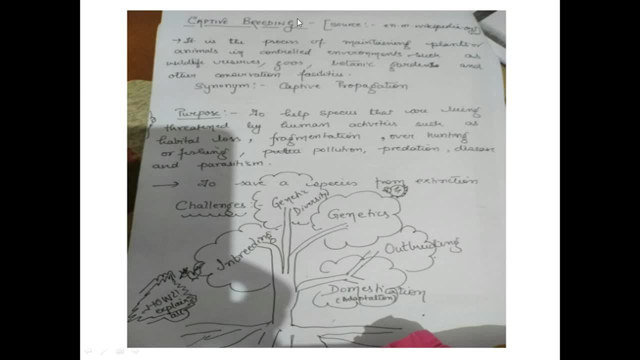 captive breeding. You all might have guessed. what is the utility of this captive breeding When you know that you need to produce large number of animals because it is supposed facing extinction, or it needs to be conserved, Or maybe because it is no more economically viable to be sustained outside you actually. 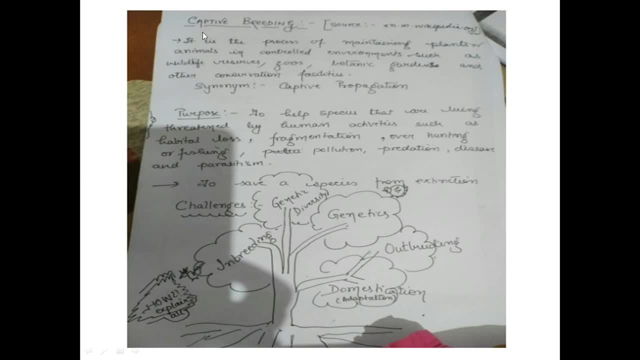 go for captive breeding and keep few of its animals. But in most of the cases, captive breeding is an important, very, very important tool to maintain the population size of an animal and to prevent it from extinction. It is a process of maintaining plant or animal in controlled environments such as wildlife. 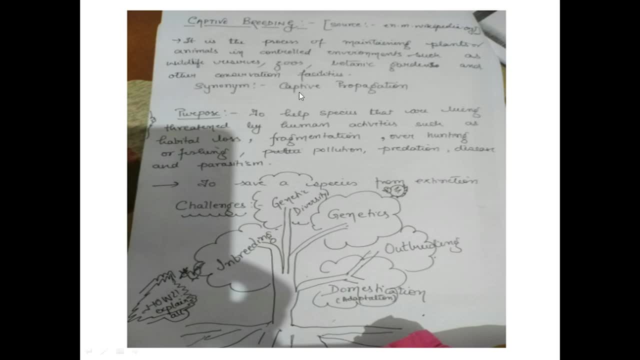 reserves, zoo, botanical garden and other conservation facilities. So it is a process of maintaining plant or animal in controlled environments such as wildlife, reserves, zoo, botanical garden and other conservation facilities. So it is a process of maintaining plant or animal in controlled environments, such as wildlife. 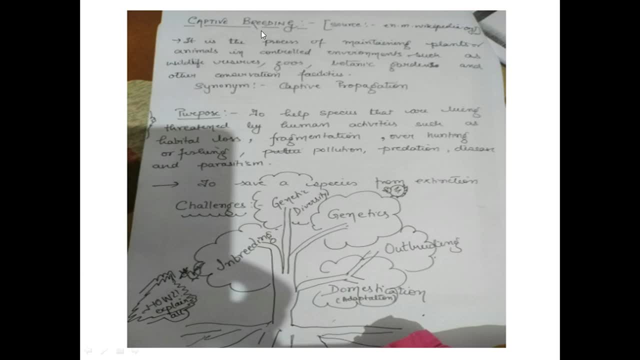 reserves, zoo, botanical garden and other conservation facilities. It's a synonymous captive propagation. So if you say, are captive breeding and captive propagation same, you will say yes, Purpose, why do we go for captive breeding? If suppose you are asked this question. If you are asked this question, if you are asked 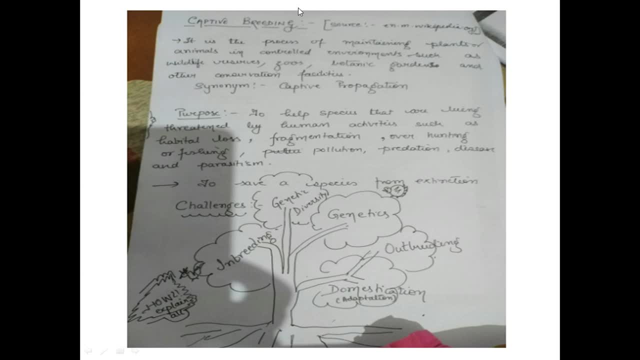 this question. if you are asked this question, the answer is to help species that are being threatened by human activities such as habitat loss, fragmentation, over-hunting or fishing pollution, predation, disease and parasitism. It means that once you have kept the animals, you have kept them for long. 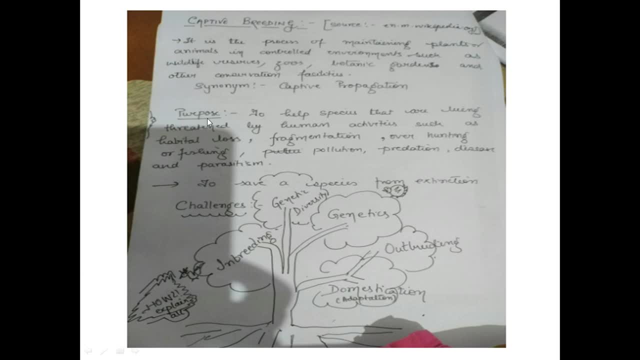 You have kept the animals, you have kept them for long. So if you have kept them for long At the time of hunting, you have kept the animals for long. species that are being threatened by human activities, such as habitat loss, fragmentation. over-hunting or fishing, pollution, predation, disease and parasitism Means for any reason. if its population size is threatened, its survivability is threatened, then you keep it in captivity separately: breed it, increase its number and leave it. 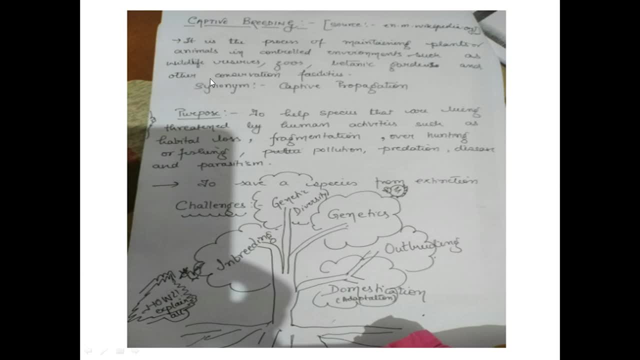 back in the wild. In most of the cases they are let into the wild again to maintain the population, to save a species from extinction. so, in nutshell, you say Now what are the challenges of captive breeding, Inbreeding? Because when you do captive breeding the genetic variability will not remain the same. 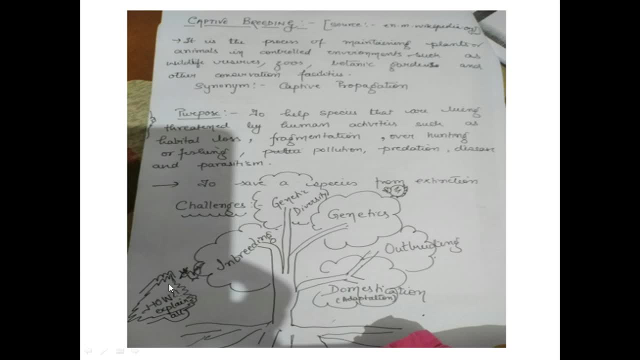 as in the wild. So there are chances of inbreeding depression. So you get a question: how Explain all So the challenges? what are the challenges of captive breeding, Inbreeding, Genetic diversity, Genetics, Outbreeding? 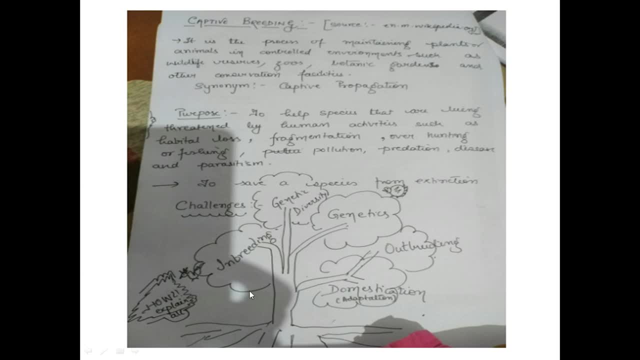 Domestication or adaptation. So these are the challenges, or constraints, with captive breeding. When you keep an animal for captive breeding, the number of animals will be decreased, and so the chances of inbreeding will be increased. Similarly, the genetic diversity is reduced, and when genetic diversity is reduced, the 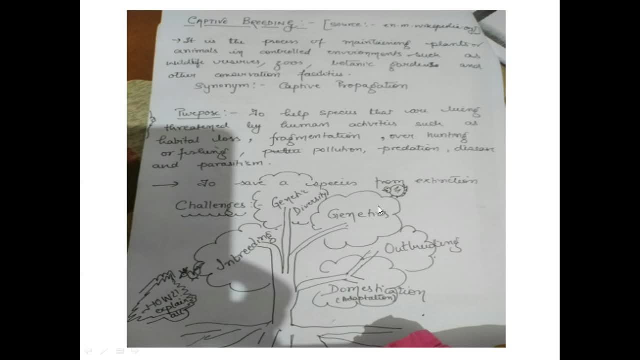 chances of heteroxys also decreases, Other reasons being genetics, outbreeding and domestication, Domestication or adaptation. A captive bred animal might not adapt when put back in the wild, or a wild animal might not respond equally to captive breeding. So these are the reasons or challenges with captive breeding. 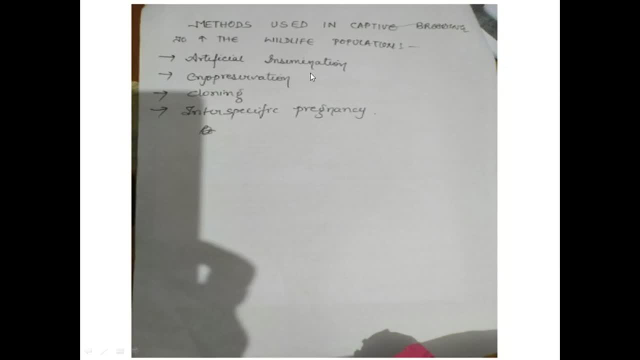 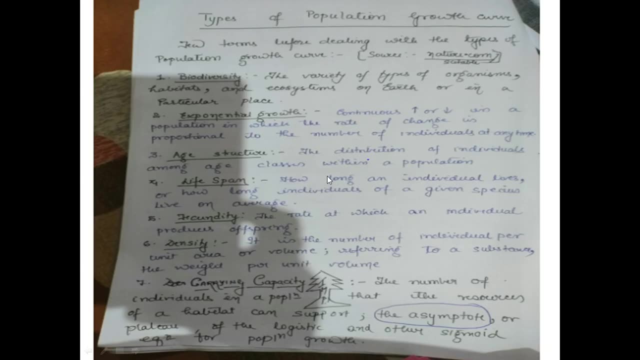 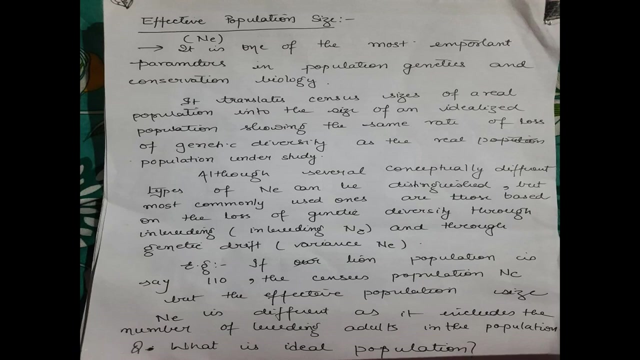 What are the methods used in captive breeding? Artificial insemination, cryopreservation, cloning and interspecific pregnancy. Now the types of population growth curve. Well, it was again: Effective population size. This is very, very, very important term. 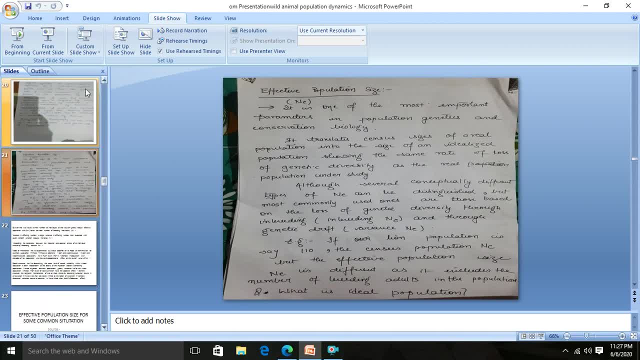 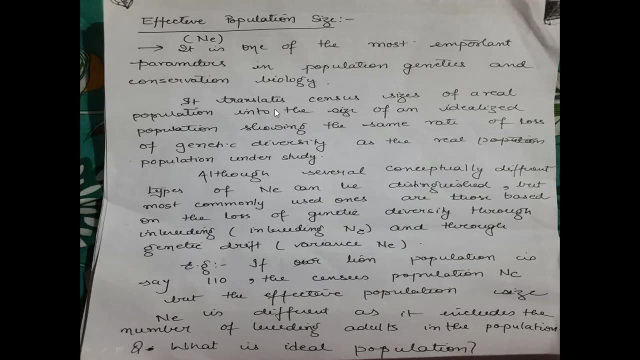 Before that, pardon me, I want to remove the two slides. Yes, they show a repetition, Exactly. Now, coming to effective population size slide show from current. It is very, very important term. Before going into it, let us discuss what. there are two terms: census, population and. 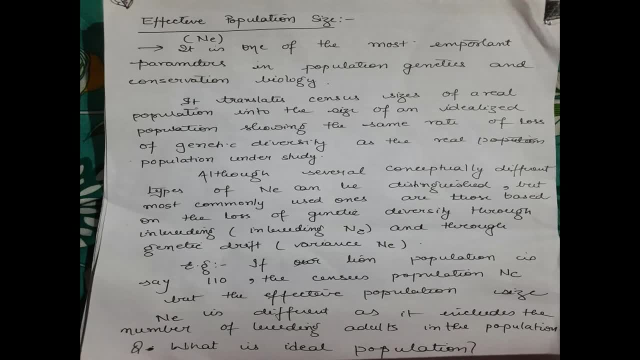 effective population size. Well, friends, they too are equally important. Census population means what we calculate through the census, From the population count or animal count, what we calculate, the total number of animals. we call it census population. But effective population size is the population size in terms of breeding which is viable. 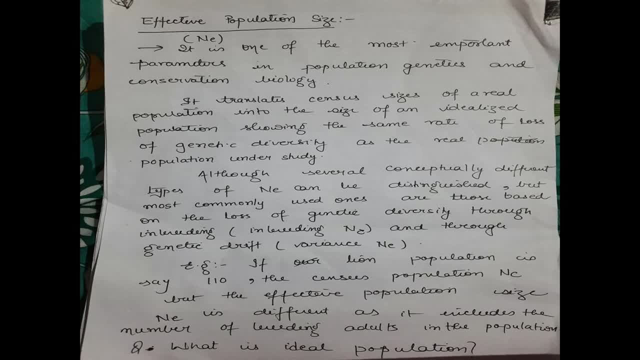 for breeding purpose Means that it is the number of population calculated on the pieces of breeding animals. It is very important because even when the census population is high, it might be at the risk of extension due to decreased effective population size. So N? E and N? C needs to be equally large for the population to not be extinct or threatened. 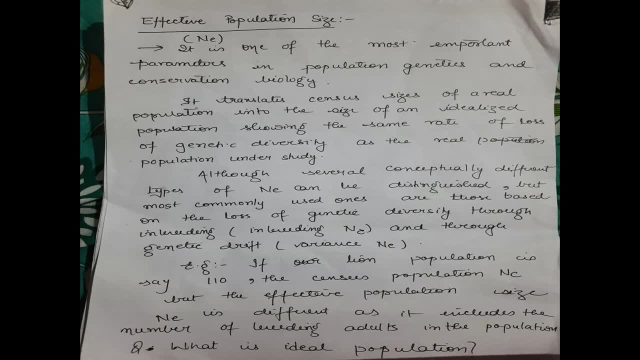 There is one thing related to this Suppose. there is such a group of animals whose population size is good. Still it has been found after studying that it is threatened or its population size is less. it is difficult for the species to survive because its effective population size is. 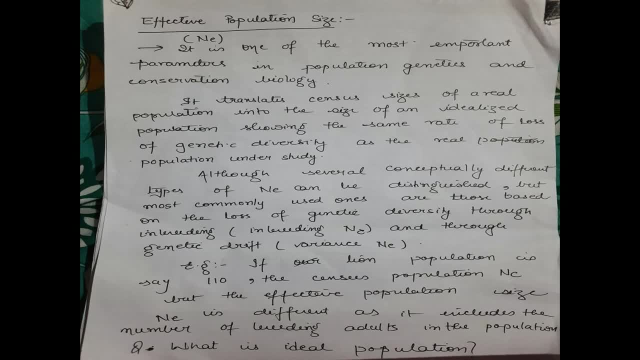 less. In other words, the numbers of males and females in that number are either more male or female. Always remember: the effective population size is approximately equal to the census population when the numbers of males and females are almost equal. You can understand the meaning of saying this way, that if there are 500 males and 500 females, 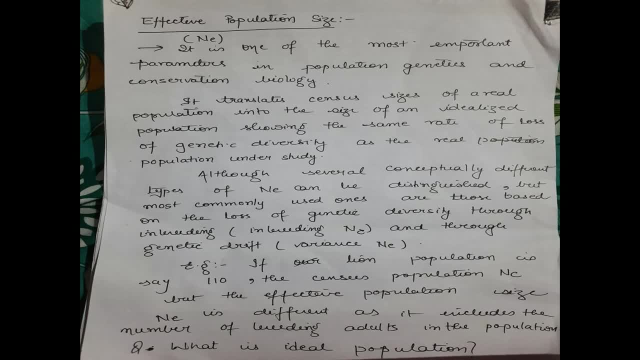 in 1000 animals. how can I calculate the number of males and females? So that is why census population is equal to the number of males and females, or 500 female hai to uske probability breeding ki jyada hogi aur isi liye uska next generation. 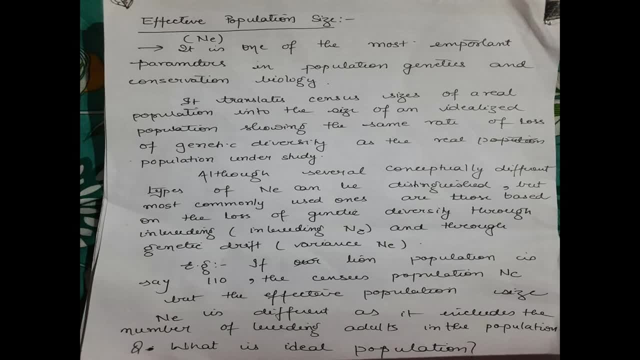 progeny jyada produce hoga. isi liye uske population size sahi maintained rahegi. say, suppose so. similarly that i'm repeating it in english- that if suppose the number of, if suppose the total population of any animal is thousand, and so if the number of male and female are exactly 500, 500 each, 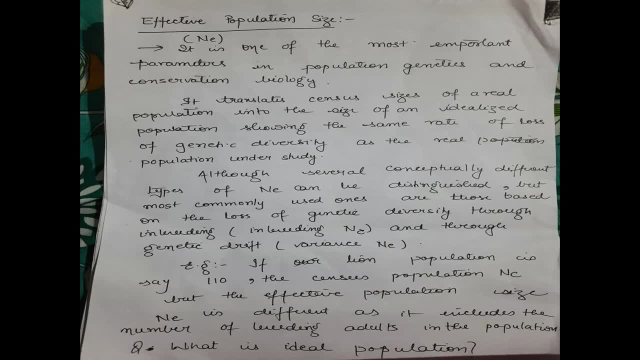 it will have maximum chances of survivability because the chances of breeding will be more among male and female and production of progeny will be more because equal number of male and female are there. so what i mean to say is that effective population size is what you ideally. 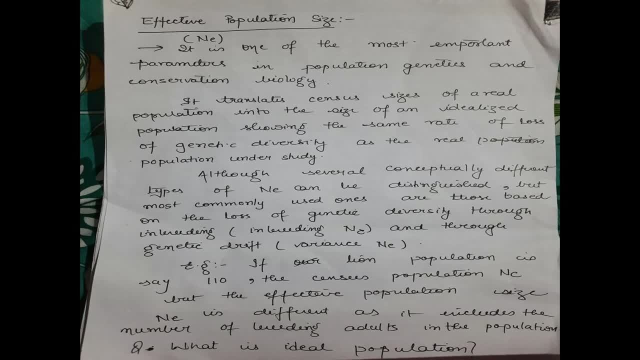 get from an idealized population of breeding animals. matlab effective population size, actually total population, ka wo. effective population size is one of the most important parameters in the population genetics and conservation biology. it translates sensor size of a real population into the size of an idealized population. 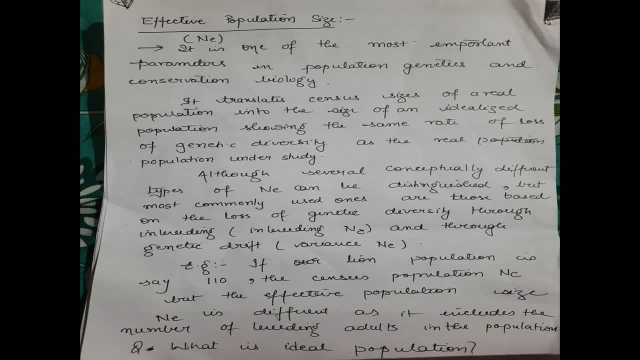 showing the same rate of loss of genetic diversity as the real population and the population under study. although several conceptually different type of any can be distinguished, but most commonly used one are those based on loss of genetic diversity in breeding and through genetic diffed variants. when we go for studying effective population size, there are two types of effective. 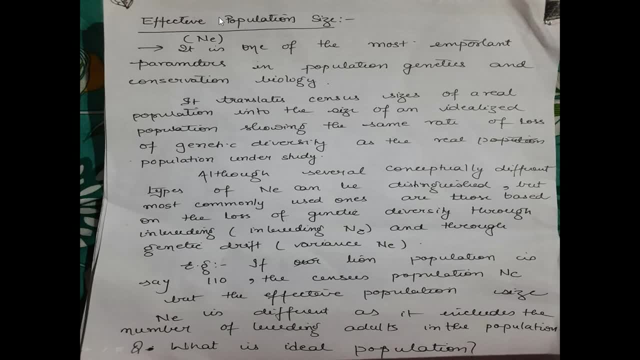 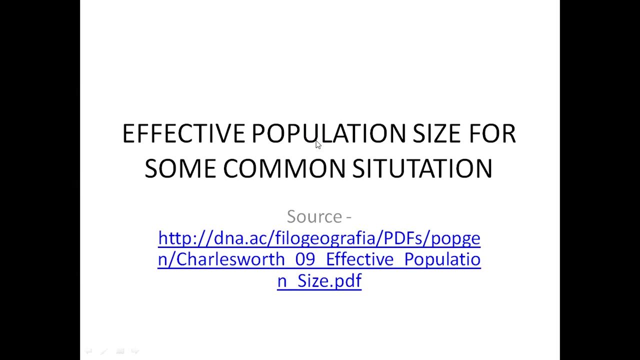 population size. we calculate effective population size on two types: inbreeding effective population size and variance. effective population size: if line in a population is 110, the census population ends say, but defective population size any is different as it includes the number of breeding adults in the population. now, in breeding effective population size, there are two types of effective population. 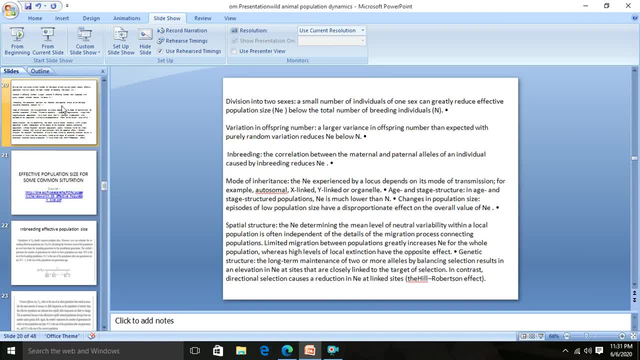 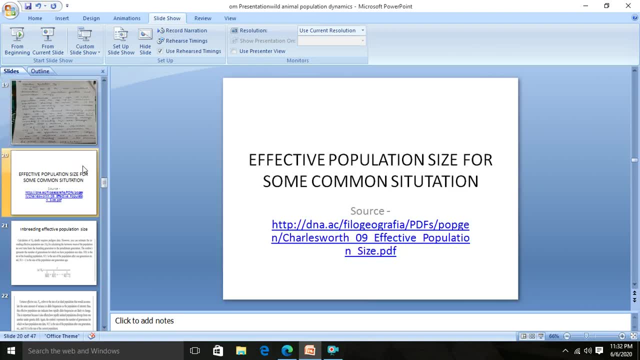 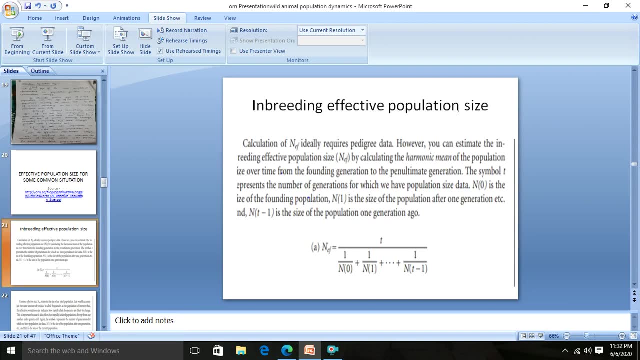 sides just a minute this: effective responses to the population size Rae, dr population size for some common situation sources as written here with due courtesy. first one is, as I told to you all, in breeding, effective population size. so just now we came to know that population sizes can be basically of two. 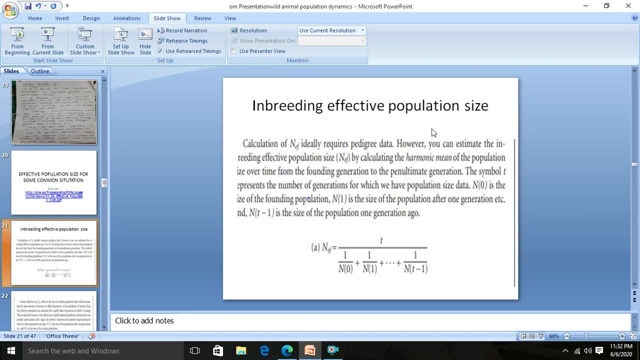 types: census population size and effective population size. then we explained that effective population size is mainly measured as of two types: in breeding effective population size and variance effective population size. coming to the first one, in reading effective population size. calculation of any F ideally requires pedigree data. however, you can estimate the in reading: 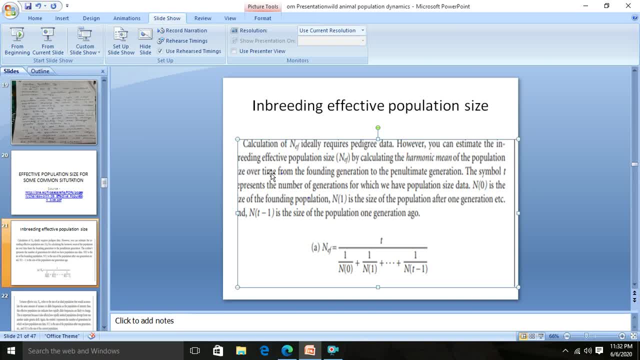 effective population size by calculating the harmonic mean of the population over time, from the founding generation to the penultimate generation. the symbol T represents the number of generation for which we have population size of the data, and n naught is the size of the founding population and one is the size. 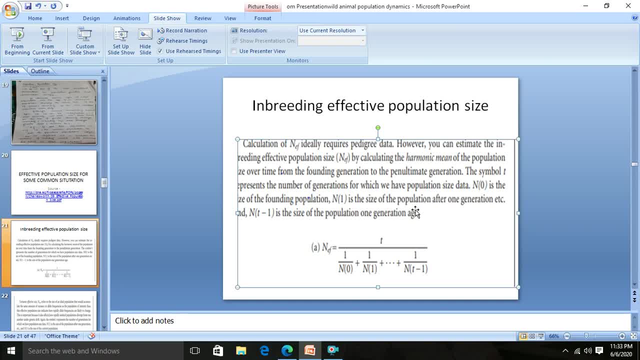 of population after one generation, and so on. any T minus one is the size of population after one generation. so if suppose in T minus one generations, you have it. suppose in T minus one generation. suppose you want to know the total effective population size on the basis of effective population size in 0, 1 and so on, up till n minus T minus one. 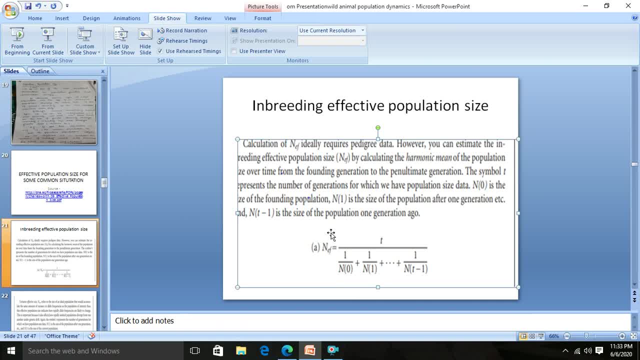 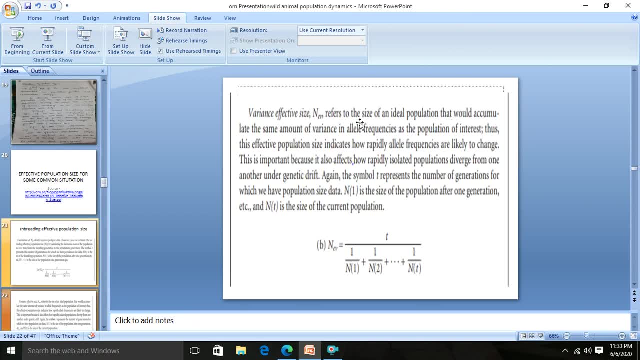 generations. so when you find the harmonic mean you get the effective population size over those generations variance. effective population size is the second type. it refers to the size of an ideal population that would accumulate the same amount of variance in allele frequencies as the population of interest does. this effective population size indicates how rapidly allele 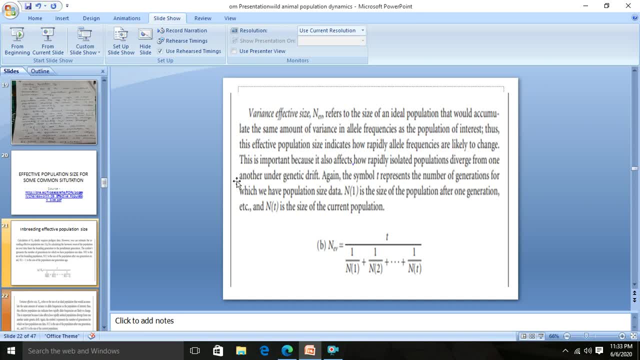 frequencies are likely to change. this is important because it also affect how rapidly isolated population diverged from one another under genetic drift. again, the symbol T represents the number of generations of which we are. populations size data. n. 1 is the size of population after one generation. 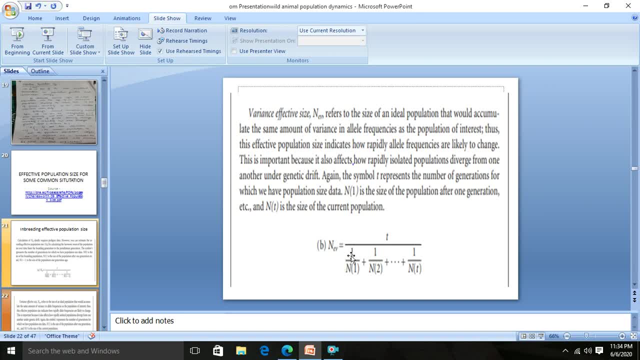 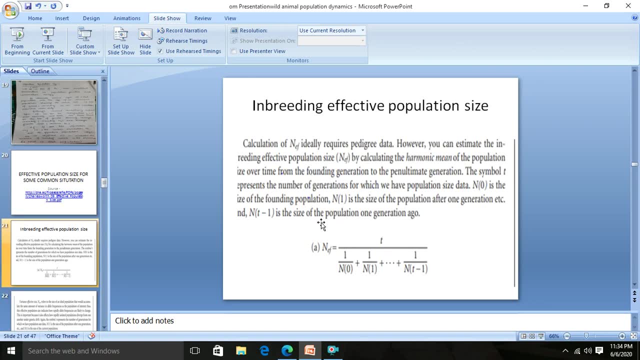 generation and NT is the size of population after current generation. This is the variance: effective population size. So what is the difference in case of inbreeding? effective population size. we take the to find the effective population size. you take the population from N0. 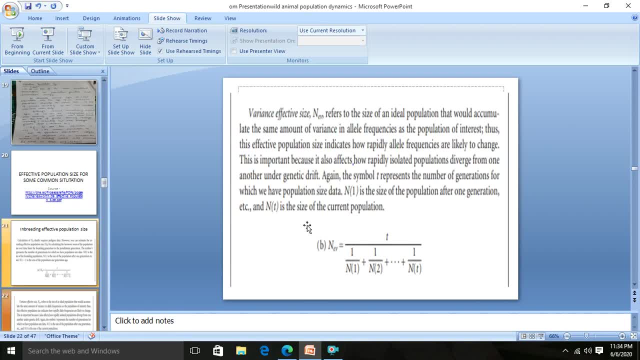 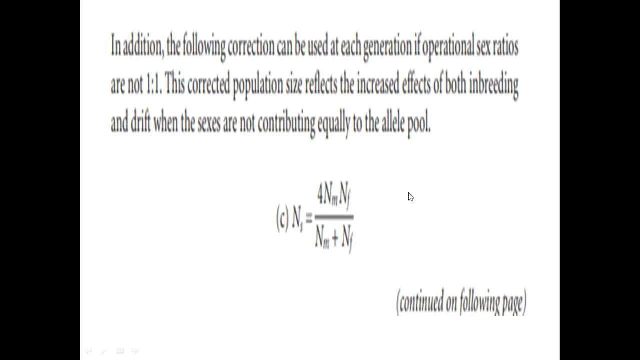 to NT minus 1 generation, while in case of variance effective population size, you take the harmonic mean from first to T generation. Now coming to the next slide, and I do it from current: yeah, this is the formula maximum used in most of the cases to calculate. it will be: 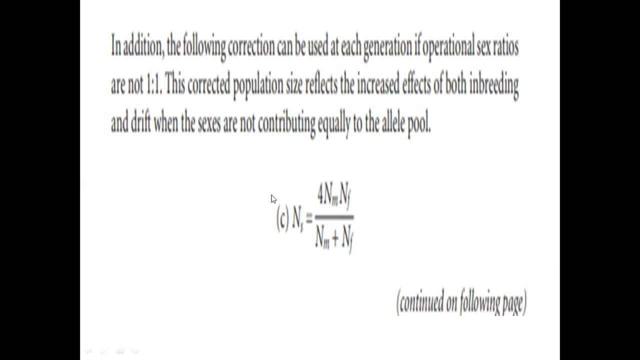 applicable for the BBSC students to calculate the effective population size, This following correction can be used in each generation. if operational sex ratios are not, 1 is to 1 and we know that in most of the cases it is not. So suppose you are asked right: calculate the. 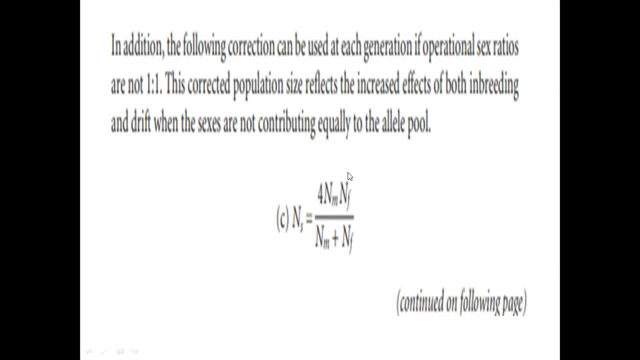 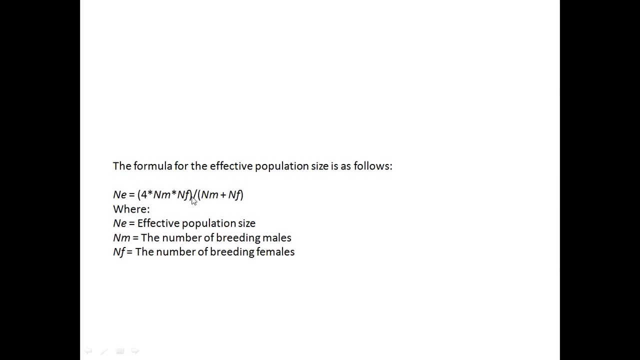 effective population size given number of generations. So you can calculate the effective population size: N is equal to 4 Nm. Nf upon Nm plus Nf. This is the formula most widely used to calculate the effective population size. N is equal to 4 Nm into Nf upon Nm plus Nf. Nm is the number. 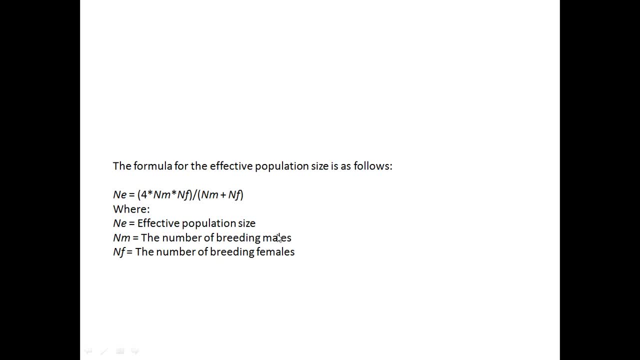 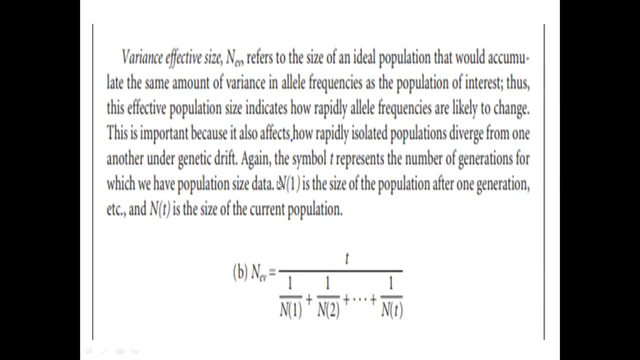 of breeding males and Nf is the number of breeding females. So you can see from this formula that if I say that this is the formula, generalized formula, although just now I taught to you all about this variance- effective population size in breeding, effective population size which you use, depending 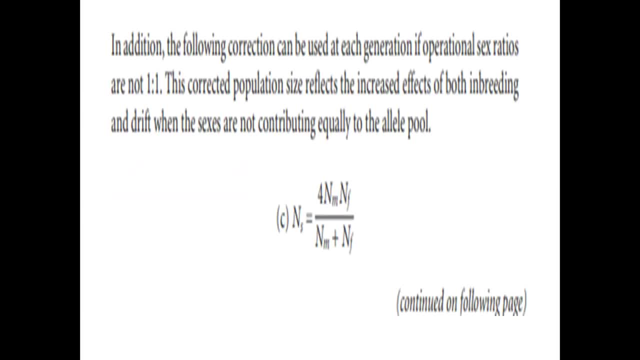 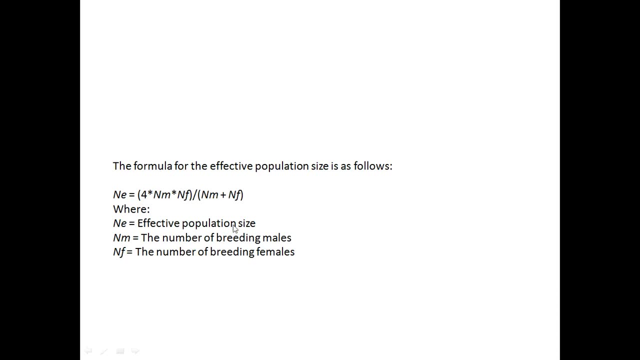 upon the data. But maximum cases for sex ratio not equal to 1 is to 1, which is, you know, is the general case. you go for this 4 Nm Nf upon Nm plus Nf. So if you are said, what is the generalized? 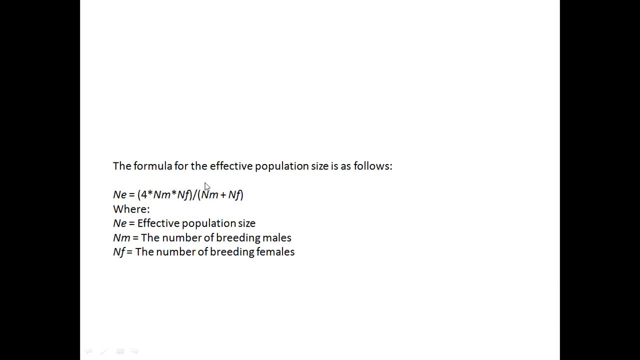 formula used, you can say this. and if you are said what are the different methods for calculating effective population size, you say all these things. Okay, so coming back to here, you can see from this formula that effective population size will be: 1 is equal to 4 Nm. Nf upon Nm plus Nf. 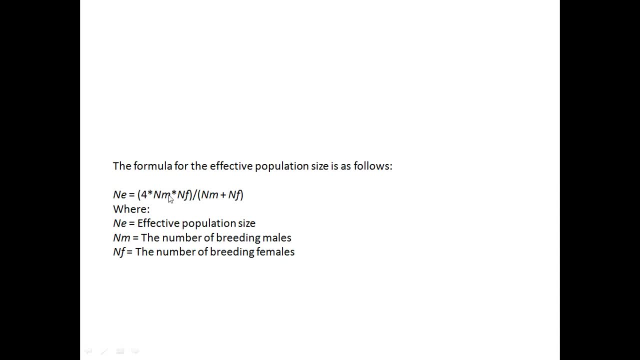 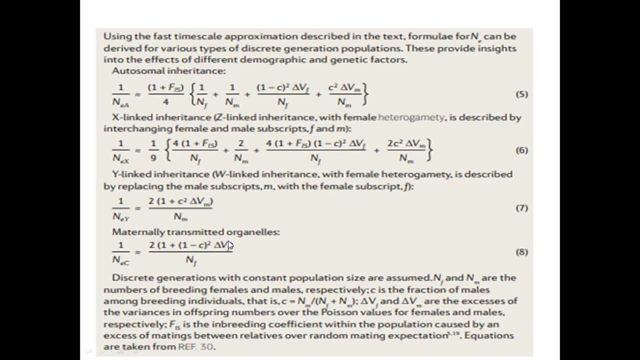 So some of these thing will be a little better. we will say less than or equal to 5 Nm, Ne will be greater. more will be the effective population size. the effective population size any will be greater for Nm and Nf being equal to each other. they are the few cases, special cases for effective. 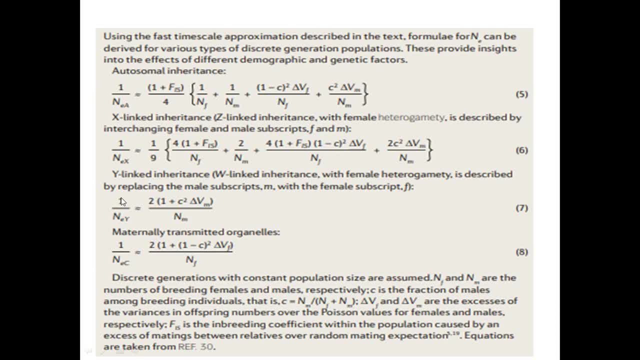 population size. this is a formula of effective population size for autosomal inheritance. this is the formula of effective population size for X linked inheritance. this is a formula of effective population size for bilinked inheritance: 29��� transmitted organelles. We do not need it for BVSC students. Now coming to the next terminology. 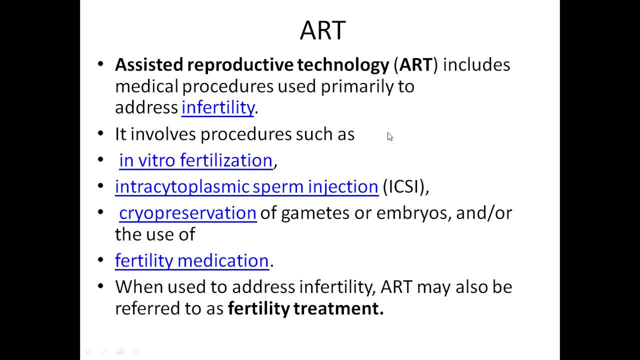 related to this wildlife populations is ART- Assisted Reproductive Terminal Technology. This Assisted Reproductive Technologies, as the name suggests, is the reproductive technology which are used to assist in the reproductive techniques to augment or to support its fertility, to increase the number of progeny, to help if support it is infertile. This ART is used. 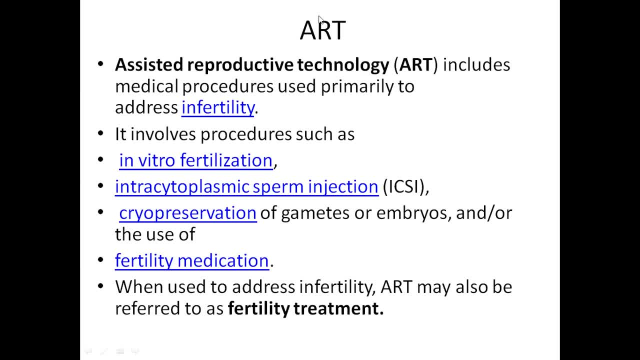 in human, in domesticated animal, in wild animals as well, to increase the number of population size, to increase the fertility and so on. It involves procedure like in vitro fertilization, intracytoplasmic sperm injection, cryopreservation, fertility medication. 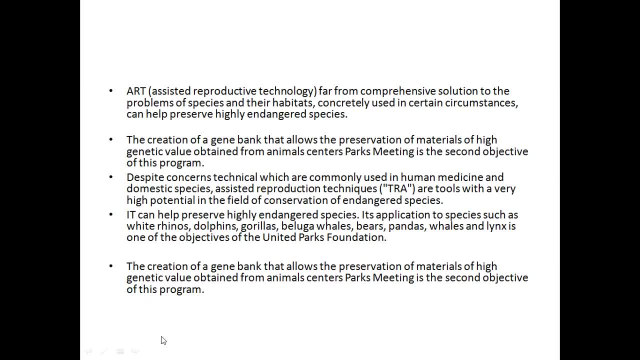 So, as you can see, this ART has limited application as far as wild animals is concerned. ART Assisted Reproductive Technology is far from comprehensive solution to the problem of species and their habitats. Concurrently used in certain circumstances can help prevents highly endangered species. 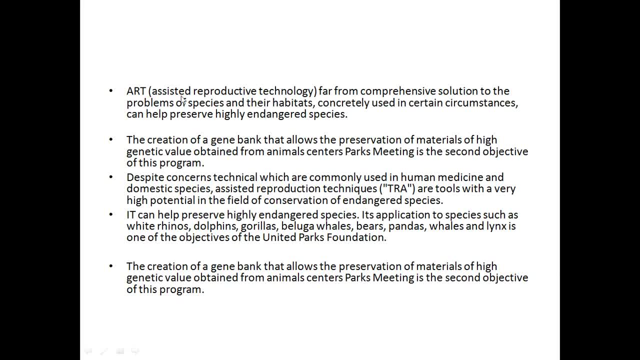 Because of its cost factor and economic viability and many other reasons, ART is rather very limited in wild animals. The creation of gene bank that allows the preservation of material of high genetic value obtained from animal centers Park meeting is the second objective of this program. 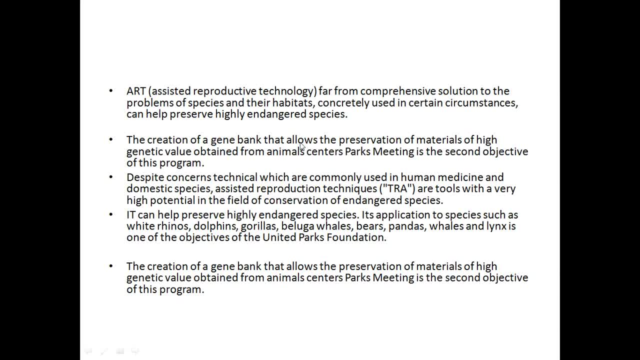 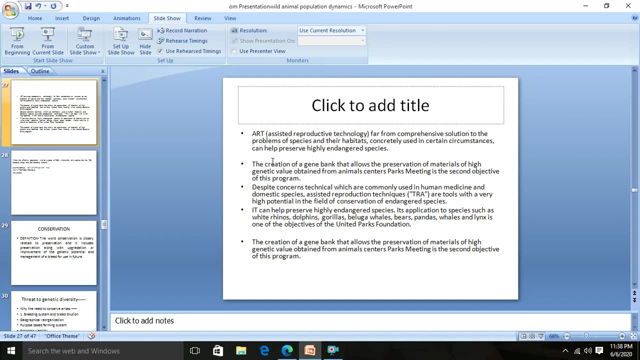 This ART was what I got from. this got from some website i must have mentioned. so this i got which showed that how it has limited resources or application in case of wild animals. this assisted reproductive technology, so it is so for the students who are online with me. students just write it in one sentence. 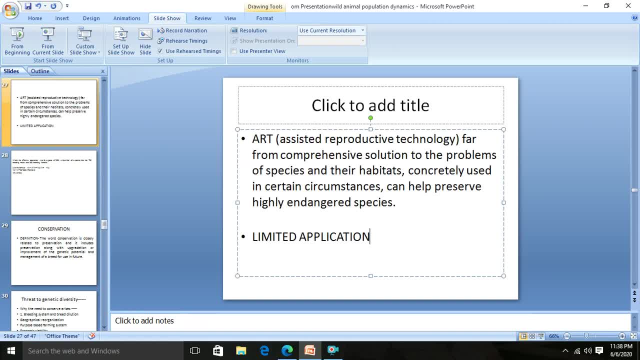 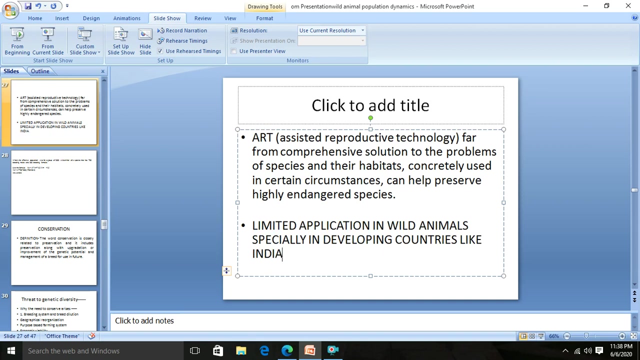 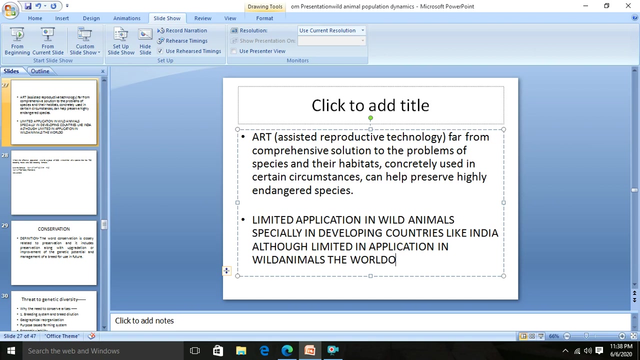 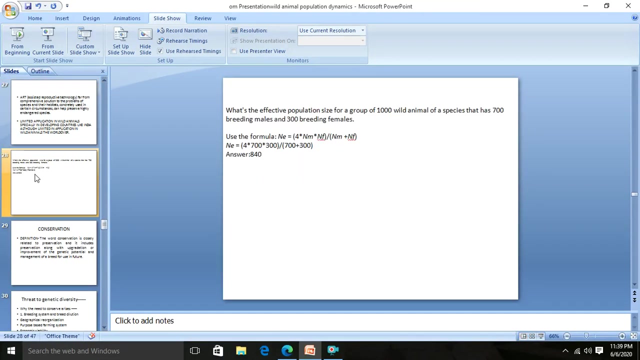 limited application in wild animals, although it is throughout the world, the condition is so, especially in developing countries like india. okay, although limited application in wild animals and is rarely used in few cases to preserve highly endangered species. fine, so again from current slideshow, but i just wanted to explain to you all what was the 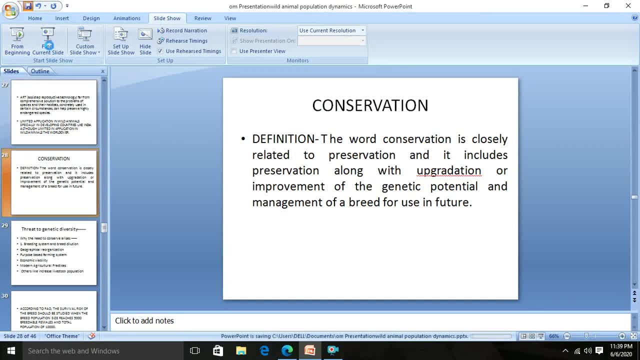 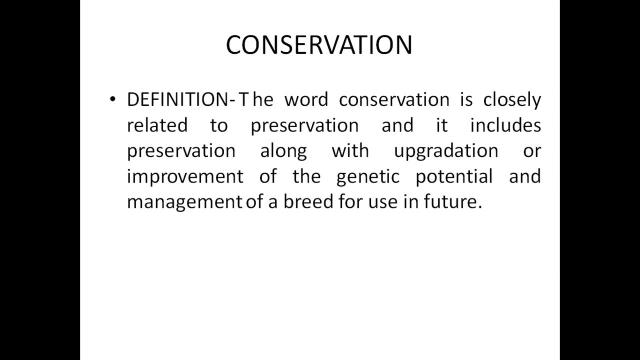 assisted reproductive technology now coming to current slide. so the next topic which will be discussing is conservation. it is very, very important topic with respect to wildlife population dynamics, as the name suggests the word conservation. let me tell you there are two words: preservation and conservation. when we keep anything as such, it is preservation, and when 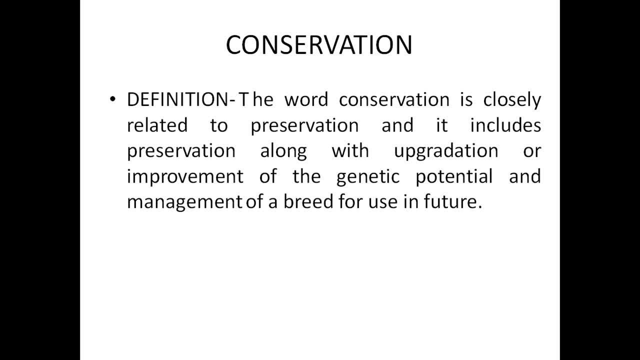 we increase it in quality or quantity, we call it as conservation. so that means that what we want to preserve is preservation, but if we want to upgrade it or increase, or increase its genetic potential, so it is not preservation but conservation. this one step, step ahead of that, so we can say that conservation is a way higher than. 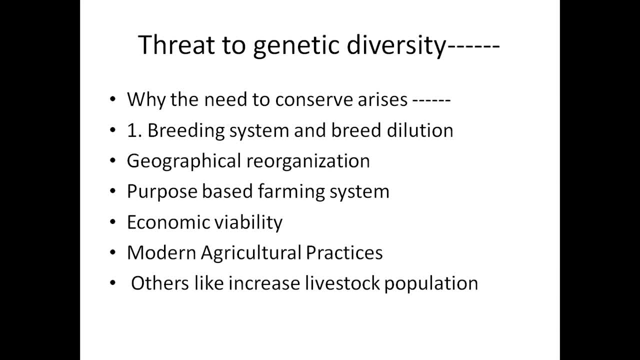 preservation now the threat of genetic diversity. why the needed to conserve arises, why we want to conserve and the need for conservation is the first thing we are looking for that to preserve and why we need it is that depends on what we want to preserve: our food and the 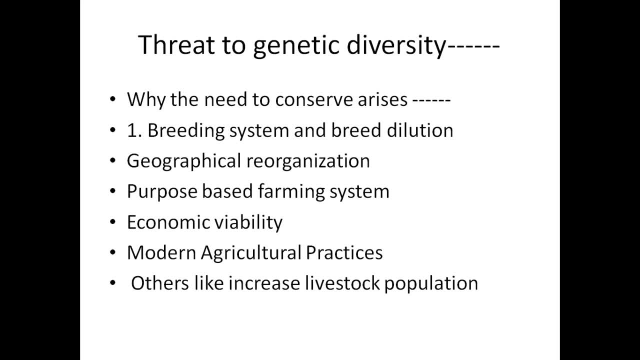 breeding system and breed dilution, geographical reorganization, purpose-based farming system, economic viability, modern agricultural practices, others, like increased livestock population Due to breeding system and breed dilutions because of methods like upgrading and crossbreeding, which we need to fulfill the demand of increasing population, the indigenous population or 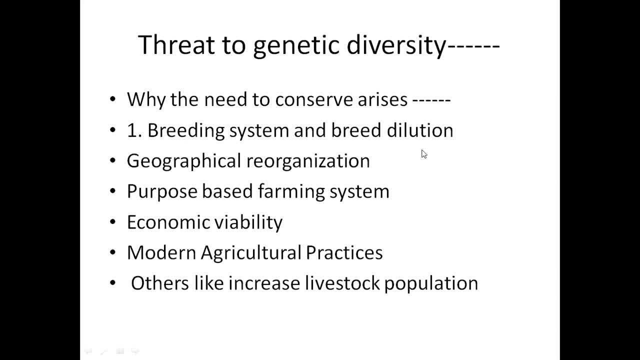 indigenous breeds are highly at threat, So we have to conserve Geographical reorganization. their habitat is disturbed many a times due to many geographical reorganizations, separation of states or nations, etc. which leads to threatening of many important breeds of animals. Purpose-based. 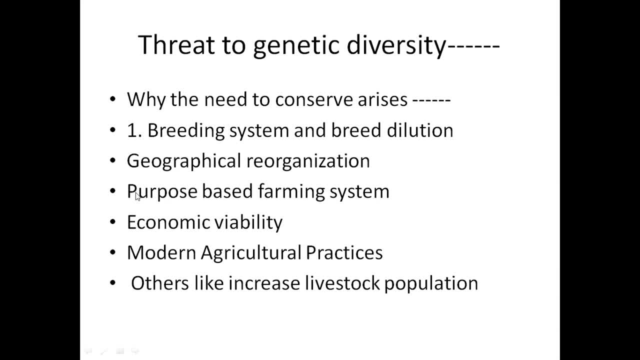 farming system, say suppose, in any area whereby no more the wool is required. so the sheep specially reared for wool will slowly and gradually start decreasing in number or threatened because it will not be reared anymore. So this is called the effect of purpose-based. 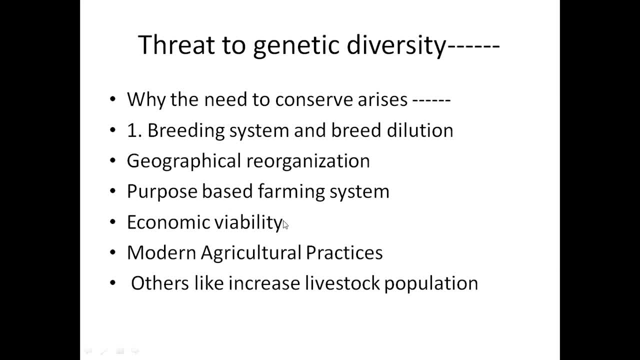 farming system. on the survivability, Now economic viability. we will not go for any desi or nondescript or indigenous animal which shows lesser productivity. Why? Because it will not be viable economically. Modern agricultural practices say: suppose now we go for tilling. 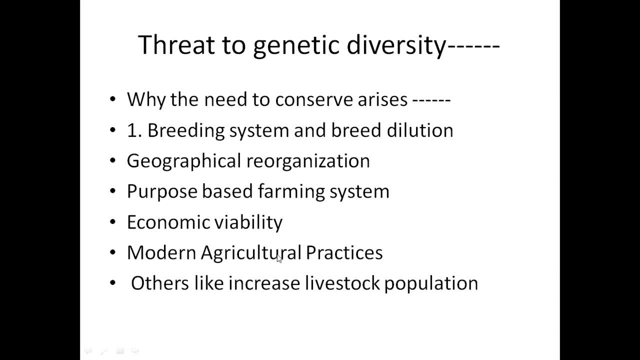 and by mechanized. The agriculture is mostly mechanized, so most of the drought animals are highly at risk or their population is endangered. So this is called as the effect. This is thus how modern agricultural practices is threatening the genetic diversity And last others, like increased livestock population, When the population increases its pressures. 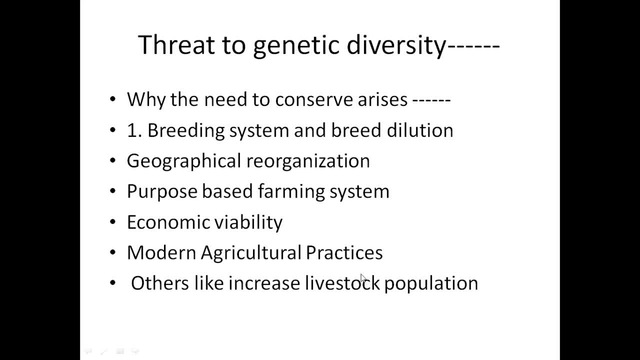 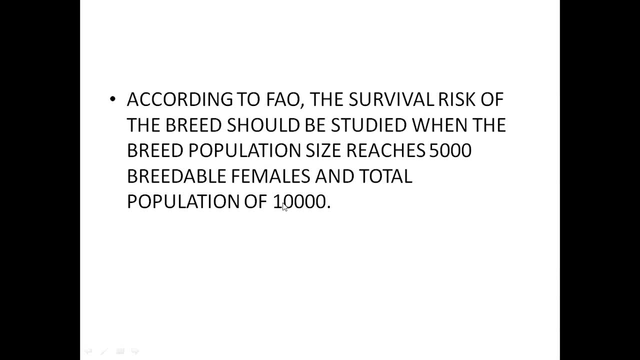 it creates a pressure, it is bound to affect the survival rate. According to FAO, the survival risk of the breed should be studied when the breed population size reaches 5,000 breedable female and the total population of 10,000. this is very, very. 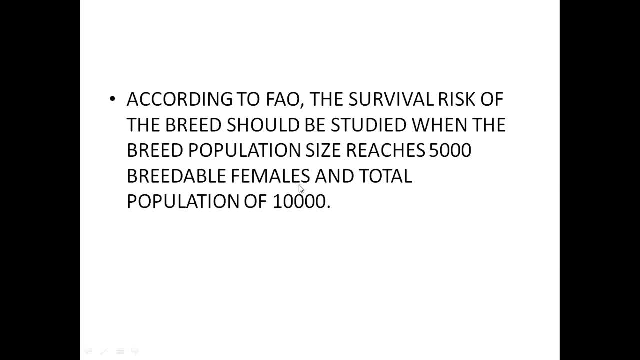 important we get in objective questions also, or multiple choice in various competitive examinations like net and all key. what if, according to FAO, the survival discovery, it should be studied when the breed population size reaches dash? it is 5,000 breedable females and total population of now. this is the data. 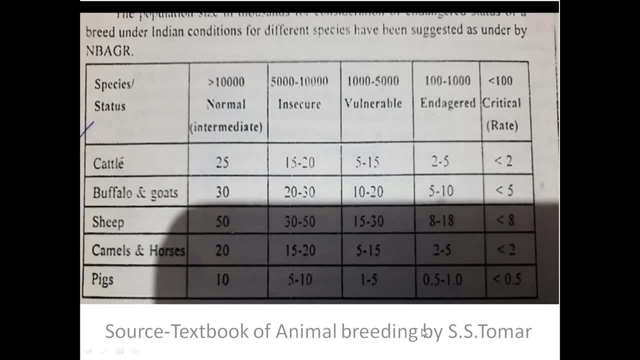 I bought from animal breeding by SS Tomer said with lot of curtsy textbook, very well, book with lot immense, I mean so much of good content. so this is where I got it. it is very important. it is a population size in thousand for consideration as endangered status of a breed, so it is the population size in. 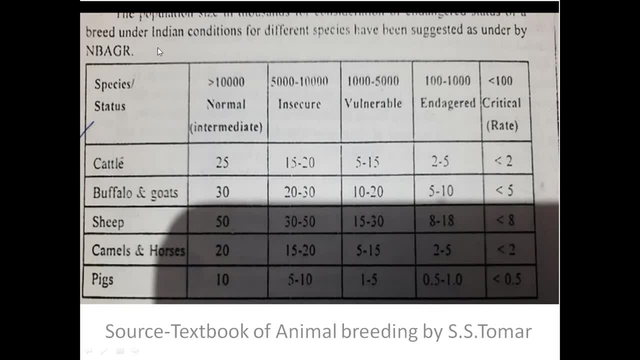 thousand for any animal to be considered as endangered species of a breed under Indian condition for different species, as suggested by NPA GR. I would like to you all to have a rough idea about it. so because you might get in different competitive examinations. so you see, in case of 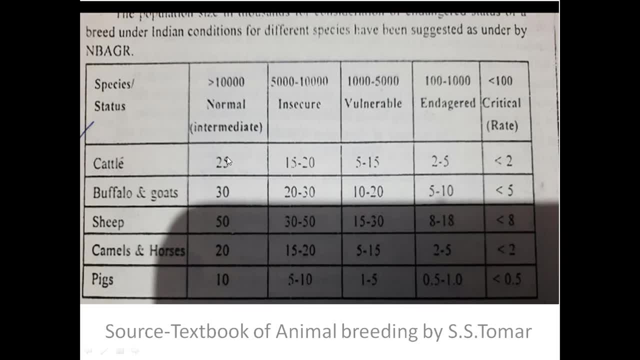 cattle it is normal when it is the population is greater than 25 and greater than so. these are the different: normal, insecure, vulnerable, endangered and critical. so you see, generally when it is less than hundred it becomes critical and in case of cattle it is called critical when the rate decreases. 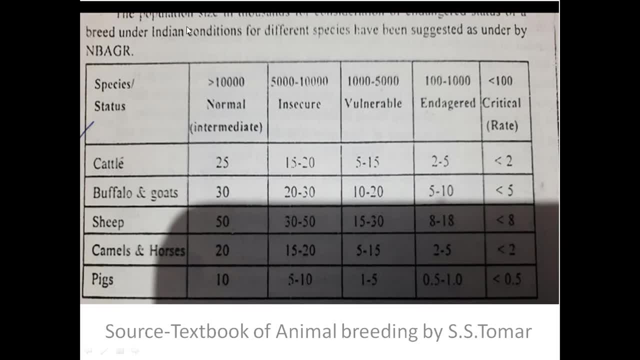 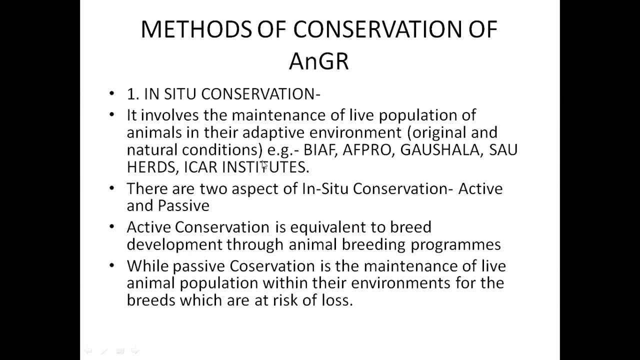 cuales udah problèmes deixan tú haas has been official to birth year. the population size in thousands for consideration of endangered status by a believed under the Indian condition. called a breed under Indian condition for different species. now method of conservation of 1920s animal genetic. 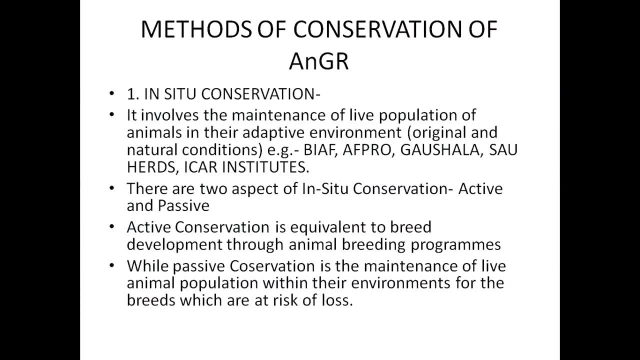 resources. there are different type of consummation. broadly it can be divided into in-situ conservation and exit to conservation. the first one, in-situ of a conservation. it involves the maintenance of life, population of animal in their adaptive environment, original and natural conditions. so when you keep the animal in their own habitat or environment, we 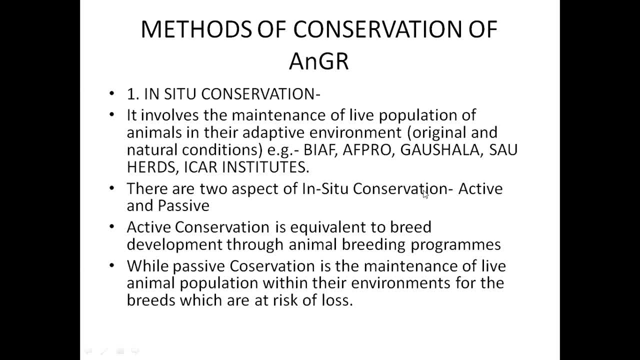 call it as in-situ conservations. so now there are two aspect of in-situ conservation: active and passive. so suppose you are trying to conserve the animals via various icr institute in the home track, maybe under different aicrp, they try to conserve it at the farmer's doorstep. it is in-situ. 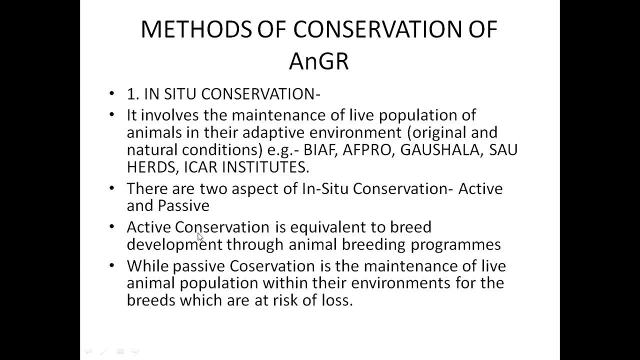 conservation. now, in case of in-situ, there is active and passive. it is further of two types. active conservation is equivalent to breed development through animal breeding program. various ngos, by, etc. also intend to increase the breed or breed develop, develop the breed through animal breeding program so they not only try to conserve it but also increase it through various 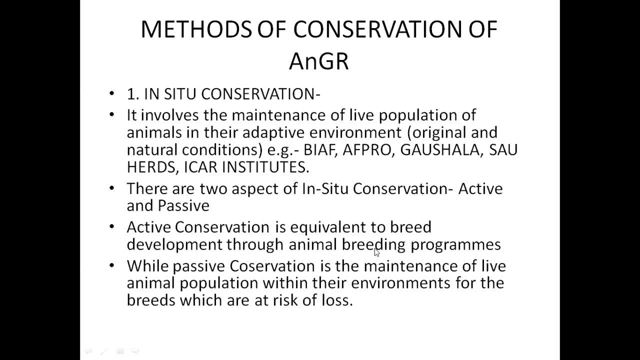 increase the potential through breeding programs so they come under active in-situ conservation, and suppose through aicrp we increase, try to increase the breed, we also do it through icrp and all and suppose through icr institutes we are just conserving it, we are not trying to increase, or 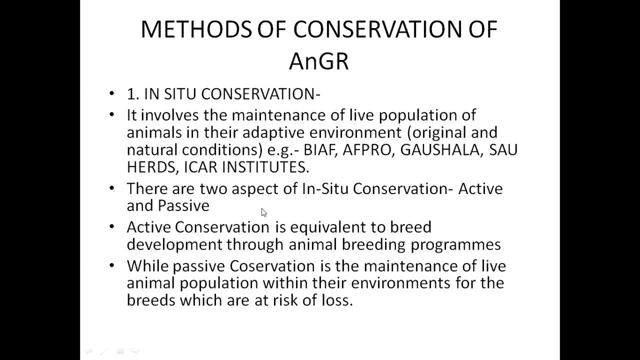 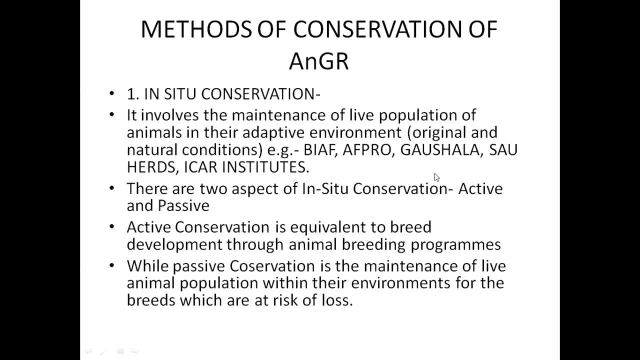 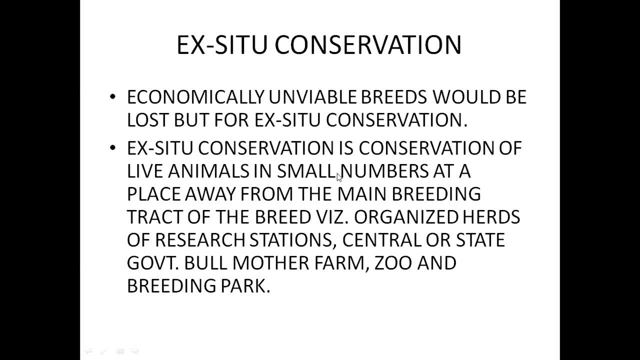 has both got to be in their adaptive environment to be considered under in-situ conservation. now coming to in-situ conservation: in-situ- ex-situ conservation- Ex-situ conservation is the second type. There are many animals which are economically unviable, and so they will not be conserved at their home track, and so they would. 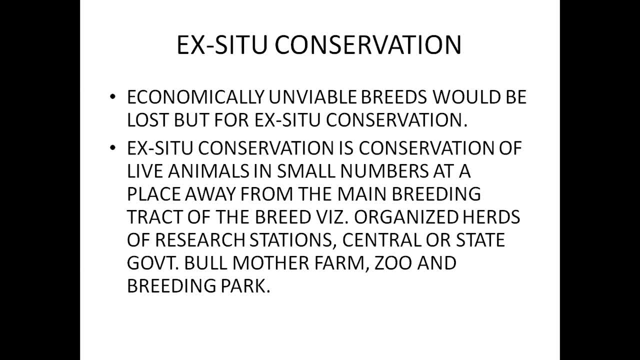 be lost if ex-situ conservation is not followed. It means that many a times the farmers, the animal owners or the farm or the herd might not be able to maintain that animal in their hometown. In that case we go for keeping the animals away from the adaptive environment for the sake of 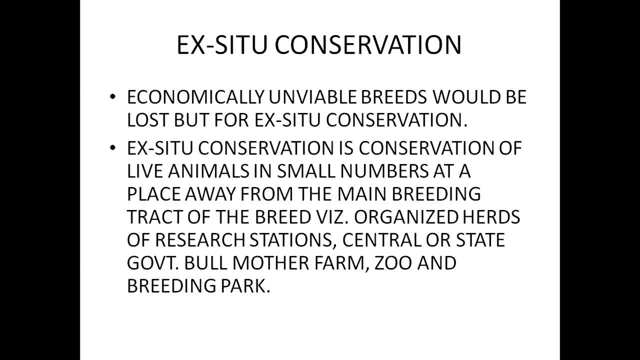 conserving it. This is called ex-situ conservation. Various all those zoo, national the parks and different type of breeding parks, like snake park, breeding parks etc. zoo, they all come under safari gardens. they all come under ex-situ conservation because there you take out the 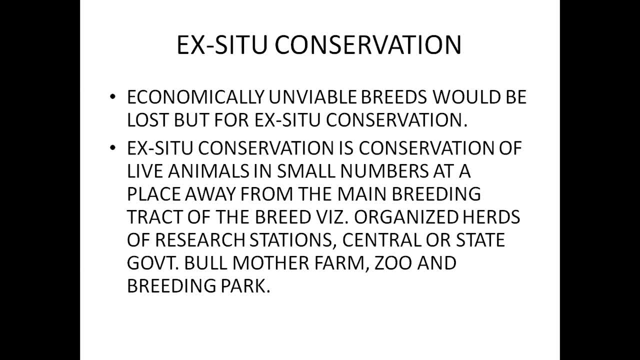 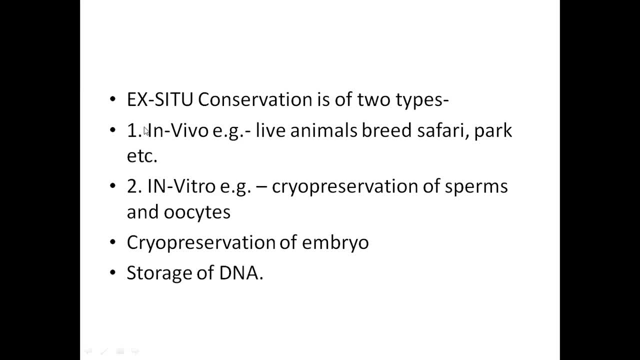 animal from its adaptive environment. You keep it somewhere else to conserve it. Ex-situ conservation is of two types further: in vivo and in vitro. In vivo, as the name suggests, in natural live animals, that if an animal is not conserved, then it is not conserved. In vivo, as the name suggests. 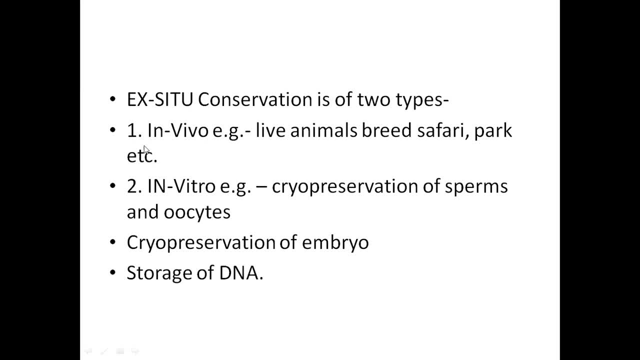 examples are breed, safari park, etc. Zoo- they are all the type of in vivo. So an important question is: zoo is an example of, so it will be in vivo, ex-situ conservation. Why? ex-situ Because it is away from its adaptive environment and in vivo because it is a live animal. The other type, 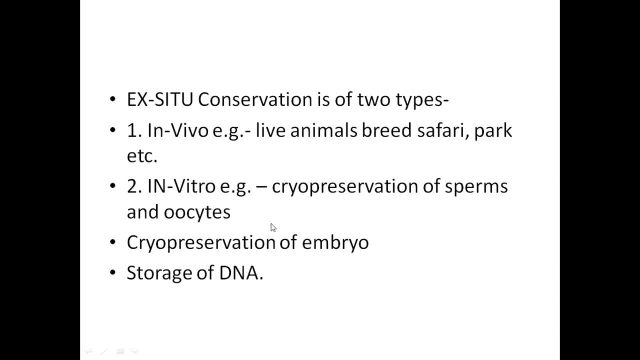 of ex-situ is in vitro. So when you go for cryopreservation that is at very low temperature- preservation of sperm and oocyte of highly precious animal, cryopreservation of embryo of highly precious animal or endangered animal- So when you go for cryopreservation that is at very low, 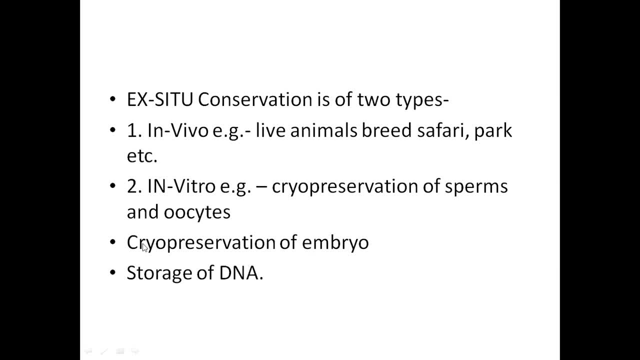 temperature. preservation of embryo of highly precious animal. cryopreservation of embryo of highly precious or endangered animal in order to conserve it, because you are conserving in either case, away from its home track, it is ex-situ. But because none of these three methods- cryopreservation. 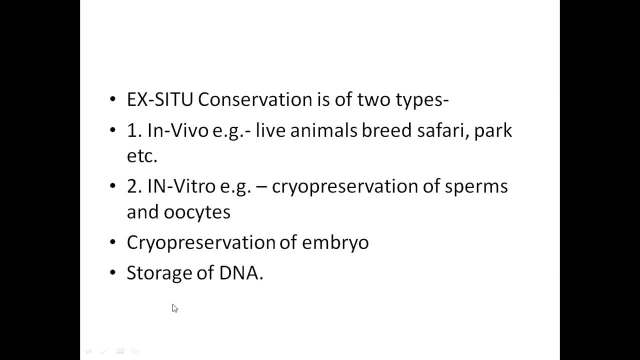 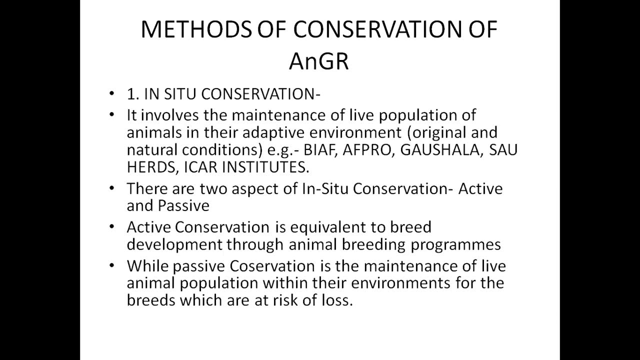 of embryo sperm or DNA is in live animal. We call it in vitro. So just now you came to know that conservation is of two types: in vivo, in situ and ex-situ. In situ is of two types: active and passive. Ex-situ is of two types: in vivo and in vitro. So in vitro. 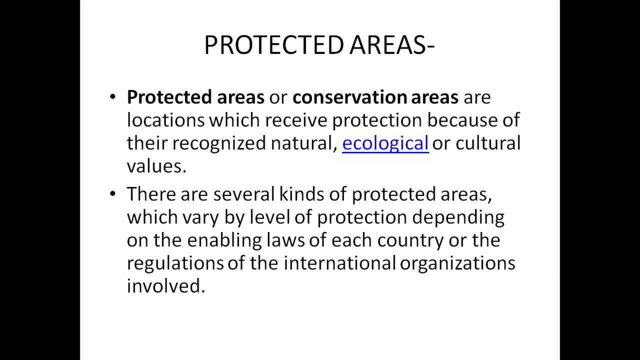 in vivo and in vitro. Last term is protected areas, As the name suggests, protected or conservation areas are the locations which receive protection because of their recognized natural, ecological or cultural values. There are several kind of protected areas, which vary by level of protection, depending on enabling laws of each country or the regulation of the. 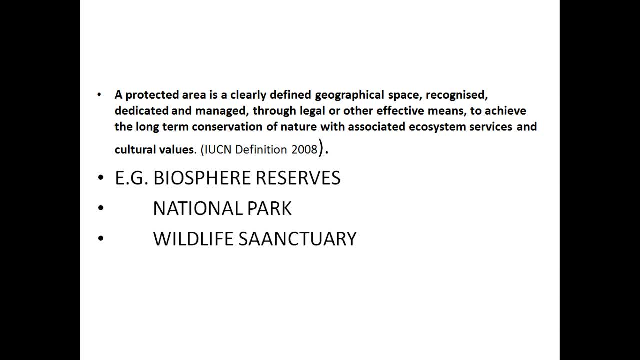 international organizations involved. A protected area is clearly defined, geographical space, recognized, dedicated and managed through legal and other effective means to achieve the long-term conservation of nature, with associated ecosystem service and cultural values. It is the definition given by 2008 IUCN. Example: biosphere reserve, national park and wildlife sanctuaries: they all 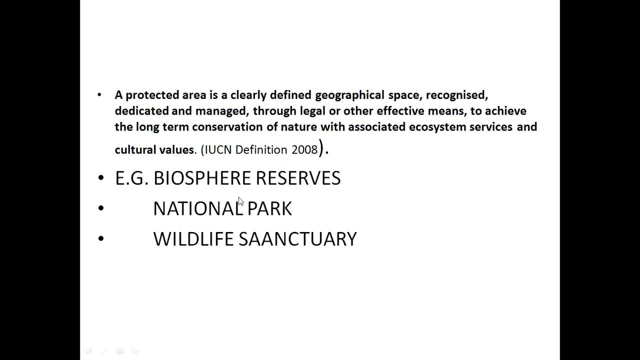 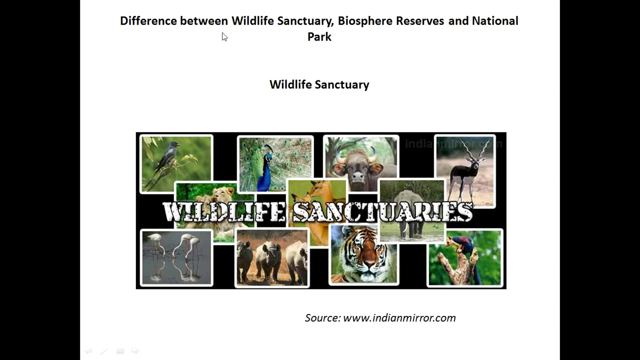 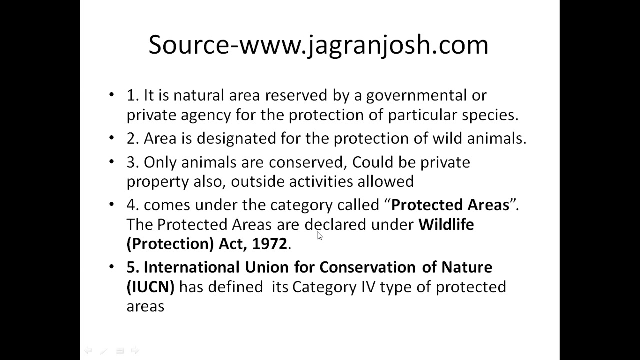 come under protected areas through clearly defined area which is considered to be partially protected, Farmers will calling that protected area. There are three types of protected areas. the first is Wildlife sanctuary: Difference between wildlife sanctuary, biosphere reserve and natural park. It is a national area reserved by governmental or private agency for the protection of particular species. 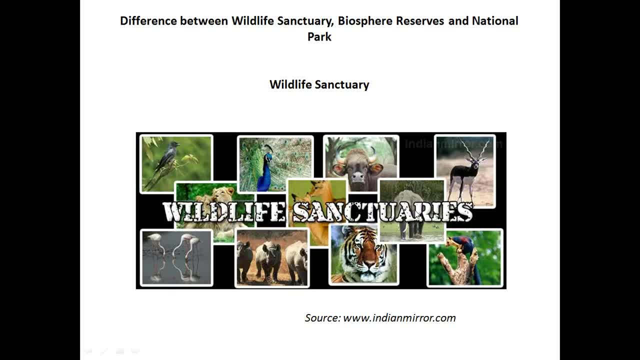 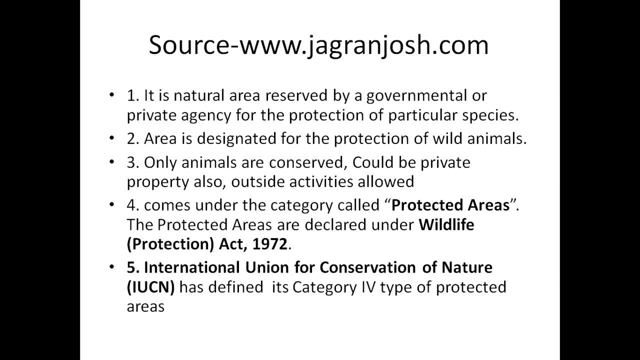 Area is designed first. wildlife sanctuary- the wildlifeтакties- is an area that the government or private agency has entitled to protect the particular species. Only animals are conserved. could be private property. also, outside activities are allowed. It comes under the category called Protected Areas. 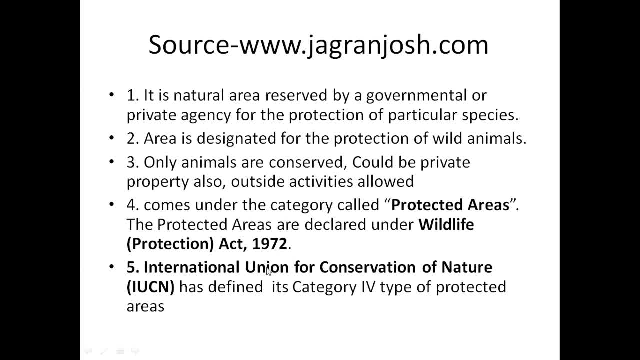 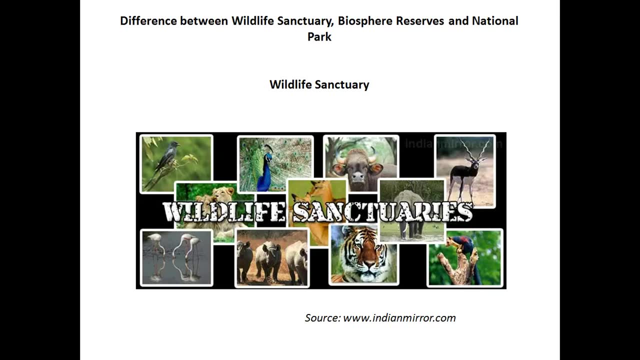 declared under Wildlife Protection Act 1972, and it is called Type 4 Protected Area. This is important. Now that we will read slowly, I will request you all to kindly compare the three, that is, Wildlife Sanctuary, Biosphere Reserve and National Park, by yourself. 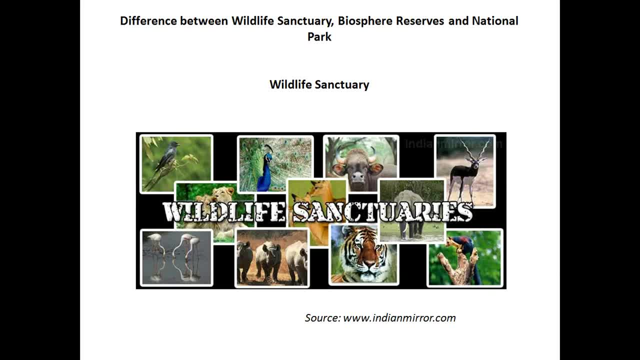 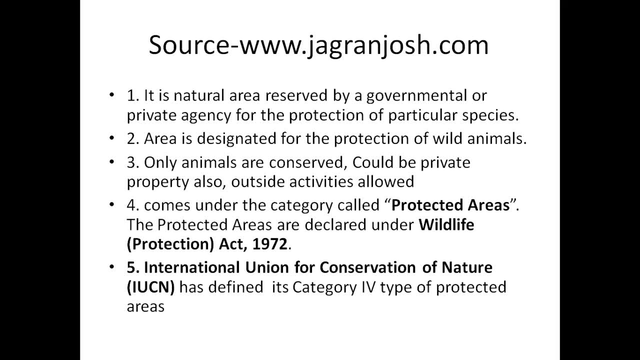 You may get a question. compare the three types of protected areas: Wildlife Sanctuary, Biosphere Reserve and National Park. Just now we are studying Wildlife Sanctuary. It is the first kind of protected area we are studying over here. It comes under Type 4 category. 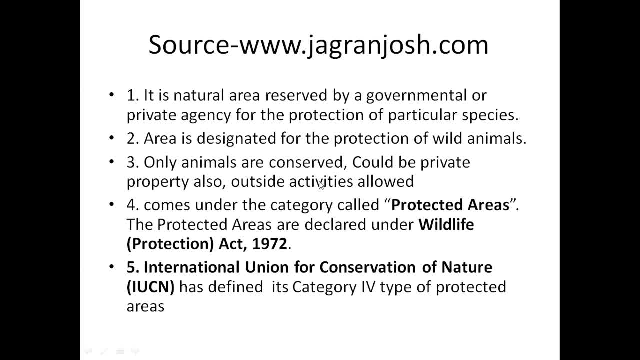 under Wildlife Protection Act 1972. In this, only animals are conserved. It could be a private property. also, Outside activity is allowed. in case of this, It is designated for protection of wild animals. Second is National Park. The characteristic of National Park is that 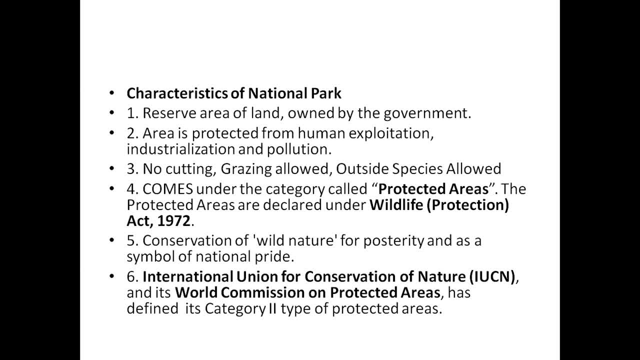 they are reserve area of land owned by government. It is protected from human exploitation, industrialization and pollution. No cutting grazing is allowed, Outside species allowed. It comes under the category called Protected Area declared under Wildlife Protection Act 1972,. 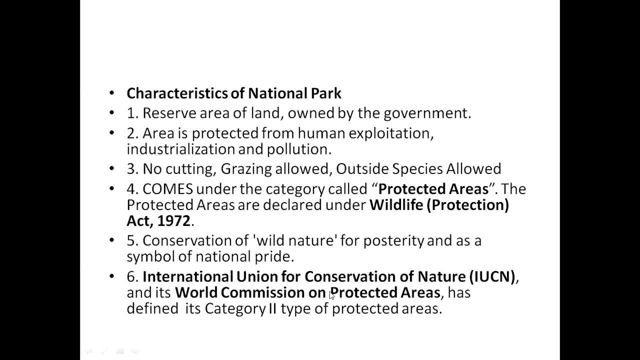 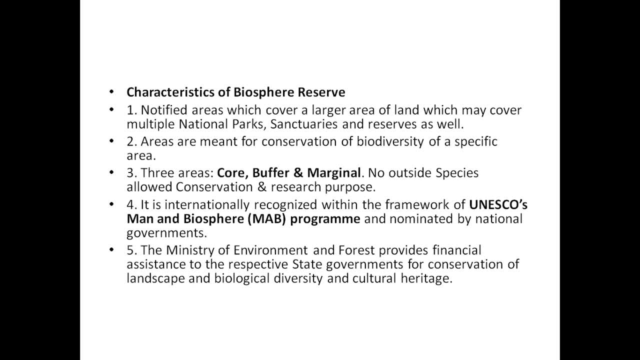 and it is of category 2.. As you have seen. so this is of category 2, this National Park, But while Wildlife Sanctuary was category 4.. Now the third one, Biosphere Reserve. The characteristic of Biosphere Reserve. 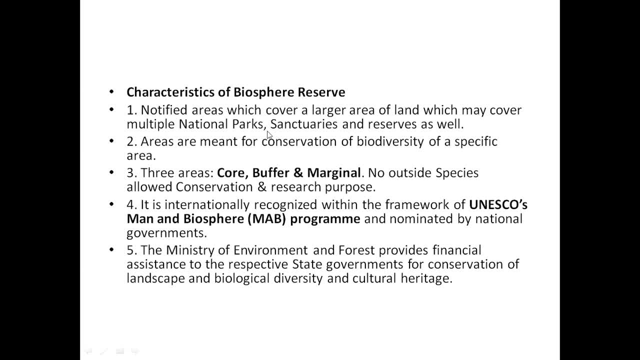 notified area which covers a large area of land which may cover multiple National Park Sanctuary and Reserve. So it is the largest of the three. That is, National Park Biosphere Reserve and Wildlife Sanctuary. Biosphere Reserve is the largest. It might cover multiple National Park Sanctuaries and Reserve. 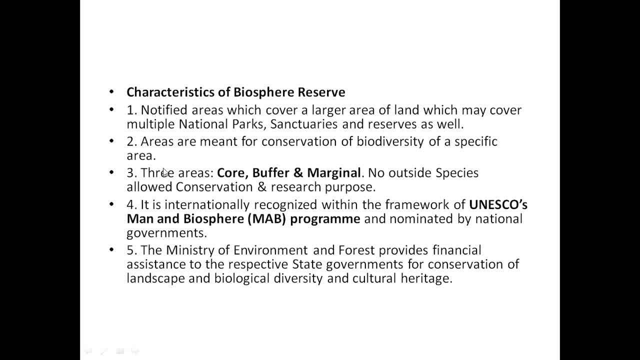 Areas are meant for conservation of biodiversity of a specific area. So it has, and it is so big in area that it has three sub areas. that is, three areas: core, buffer and marginal. No outside species allowed. conservation and research purpose is only there. 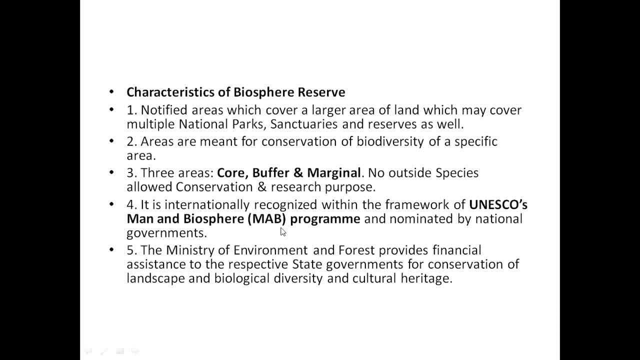 It is internationally recognized within the framework of UNESCO Man and Biosphere Program Very, very important. The Biosphere Reserve out of three is recognized under MAB Program. The other two, Wildlife Sanctuary and National Park, are not. The Minister of Environment and Forest provide financial assistance. 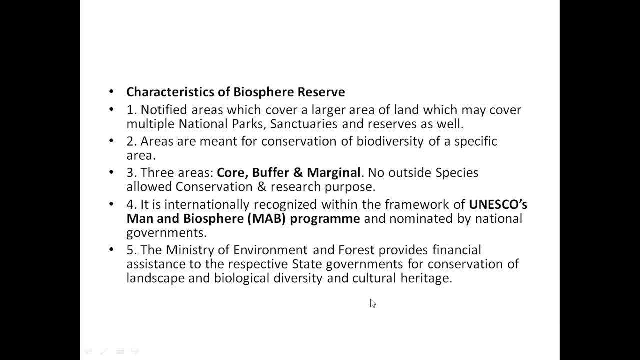 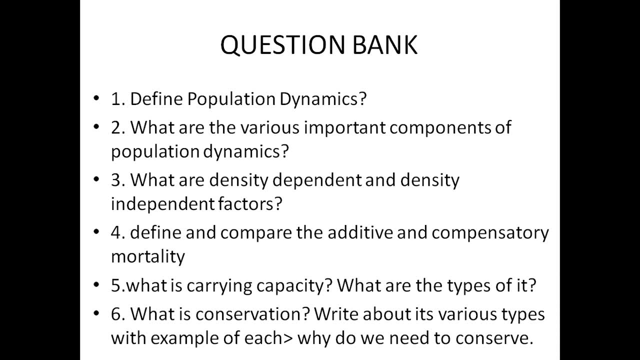 to respective state government for conservation of land spec and biological diversity and cultural heritage. So this is the question bank. based upon what I taught today, I request you all to try solving it. They are all been dealt in the lecture. This lecture was especially meant for the wildlife population dynamics.